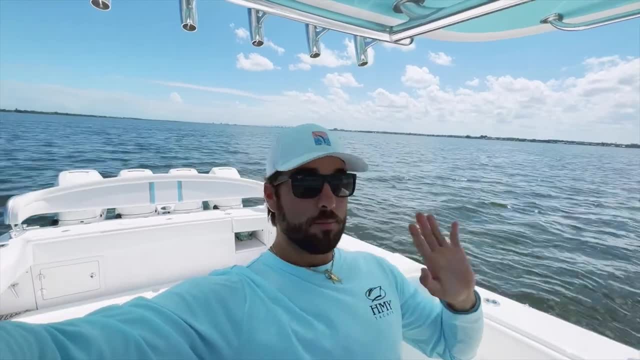 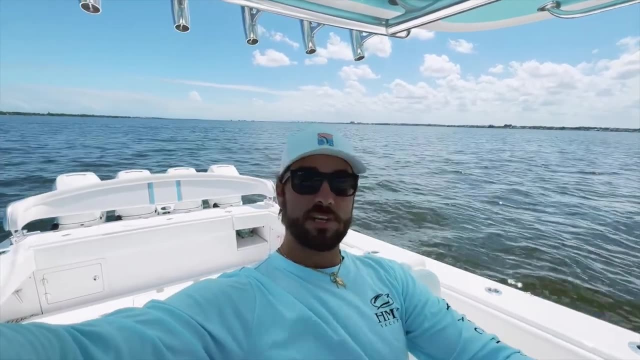 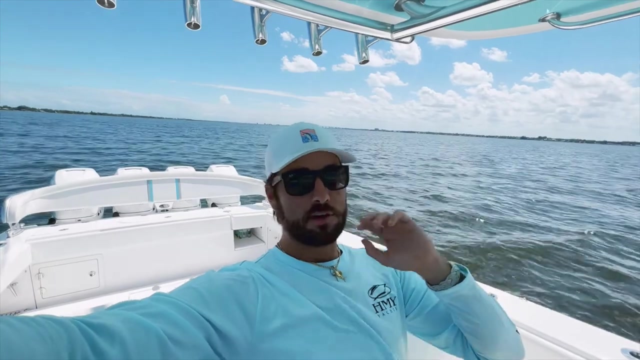 minimum age. I could be wrong double check, but I believe as long as you can pass the exam, you're good and you can go out. you also do have to have a government-issued photo id- a valid one- with you along with that boater safety card. certification card looks like a credit card. 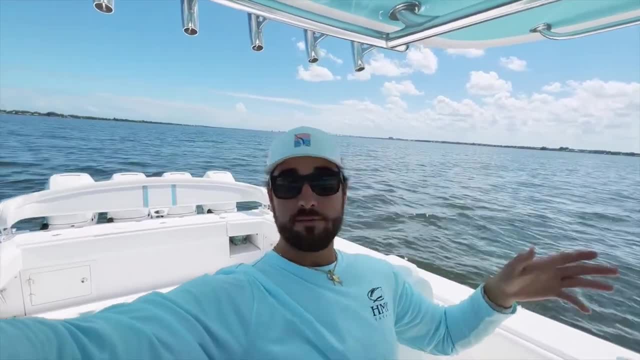 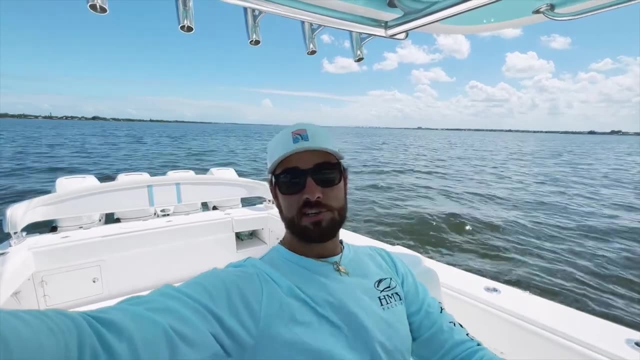 you have to have both of those things and you can be able to get into a boat without a safety card out, go rent a boat, do whatever you want and drive a boat around. now, if you own a boat, there's a couple extra steps. that boat has to be registered in your state here in Florida. if you want to own a boat, you 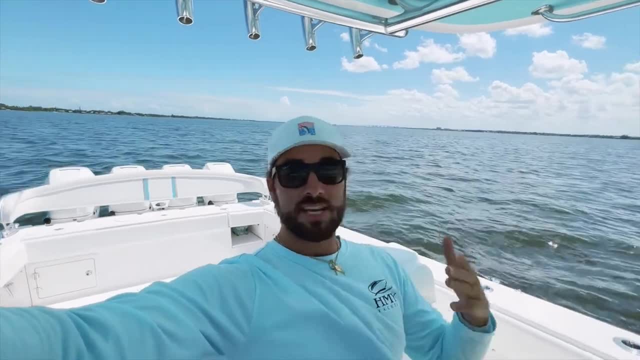 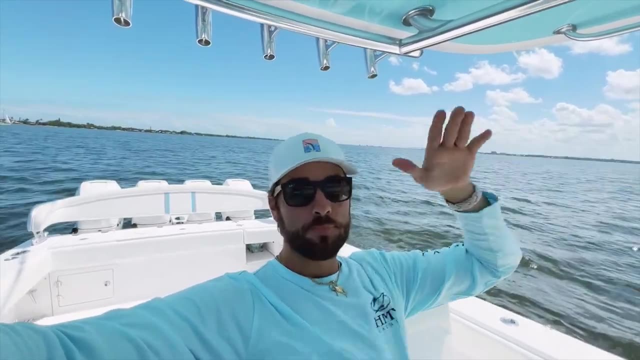 have to register it and pay your state taxes, and so when you do that, you get a bunch of paperwork and then you're given a number and that number has to be visible on the on the hull side, towards the bow, along with your registration sticker. and that's for very basic boaters. chances are anyone 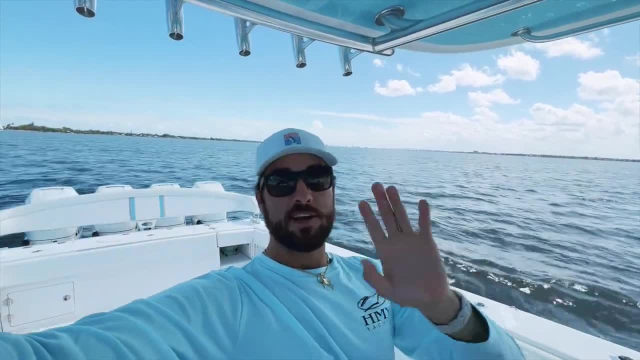 watching this video is not going to document their boat registration. This video is not going to document their boat registration. This video is not going to document their boat registration. this video is not going to document your vessel, which i'll talk about in a second. 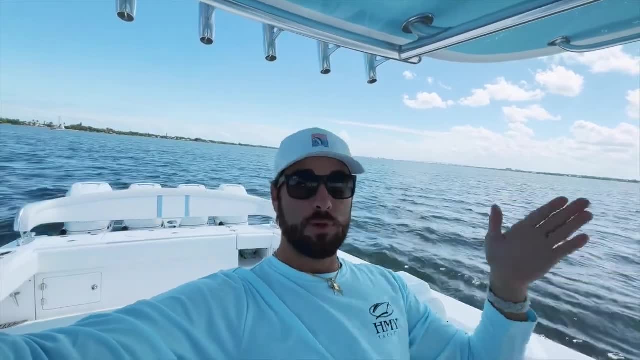 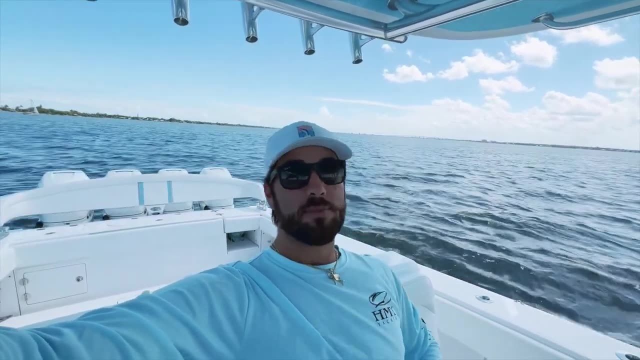 and if you do not document your vessel, you need to have those numbers visible on your bow along with your registration sticker. now you do have the option also to document your vessel with the us coast guard, which is just an additional step. it gives you some protections if you plan on. 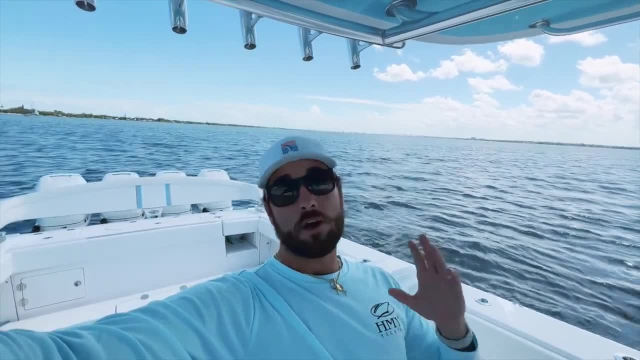 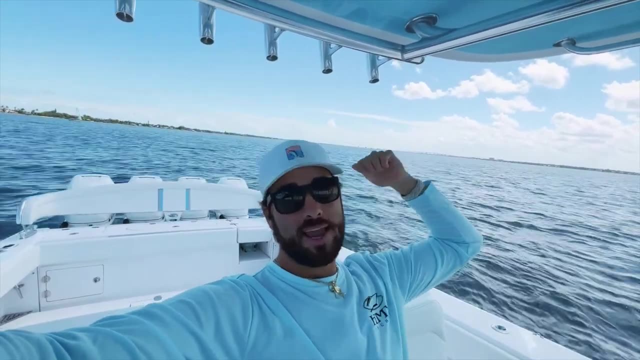 you know, going in international waters, all that kind of stuff, and what it also allows you to do is to not have to put your numbers up on your bow, as long as you have the name of the boat and the hailing port on the transom of the boat, and there are some of these numbers that are 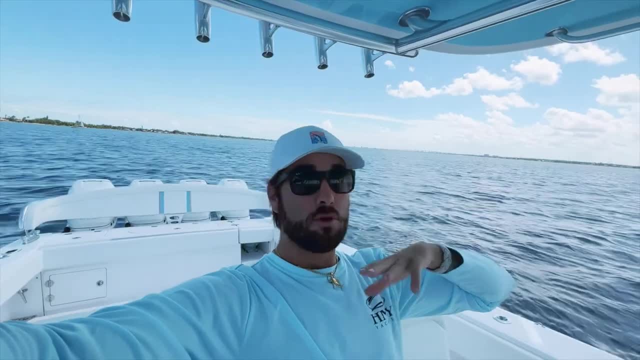 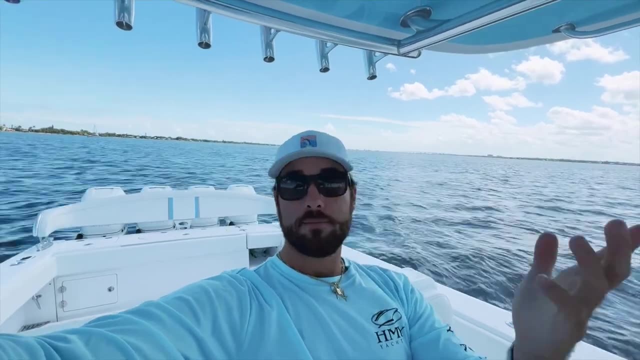 some regulations on size, but as long as you have those on the transfer on the boat, you do not have to have the numbers on your bow. you still have to have the registration sticker somewhere visible on the boat. you know this boat is documented, so we have the name on the back and i'll show you here. 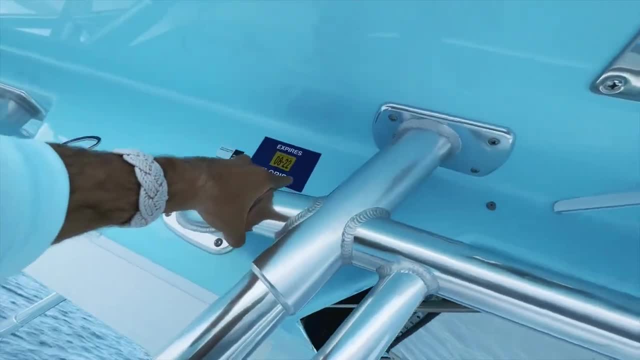 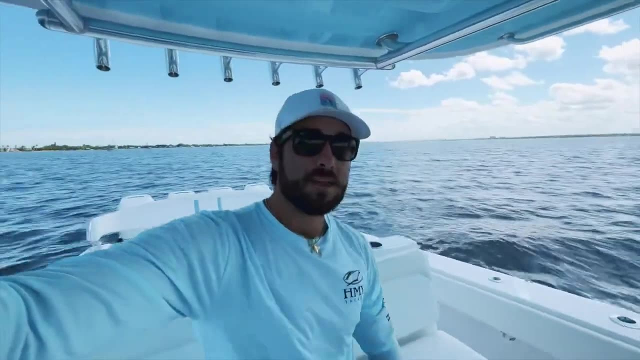 our registration sticker is on the top top of the t-top right here, which it actually is expired. i have the new one at home, i just haven't replaced it, but that's the minimum of what you have to do to make sure your boat is legal to be in the waterways. um, that's pretty much it when it comes. 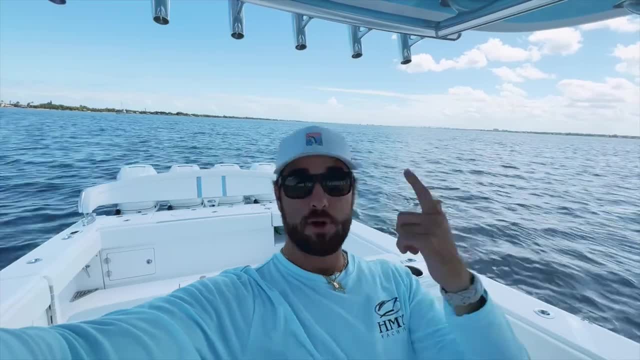 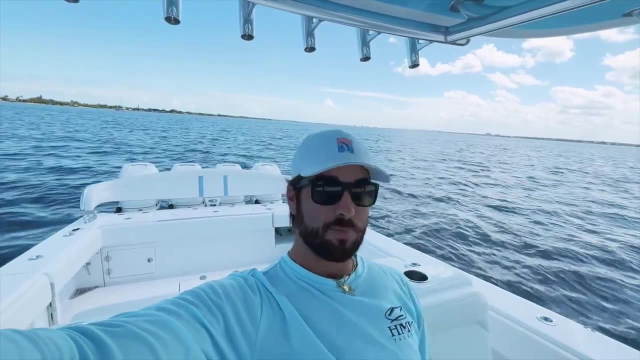 to the the government regulations. all you have to have from that is your boater safety card and id, to go along with that the photo id, and then make sure your boat is registered and taxes are paid in the state you want to use the waters, assuming you are a us resident and the boat 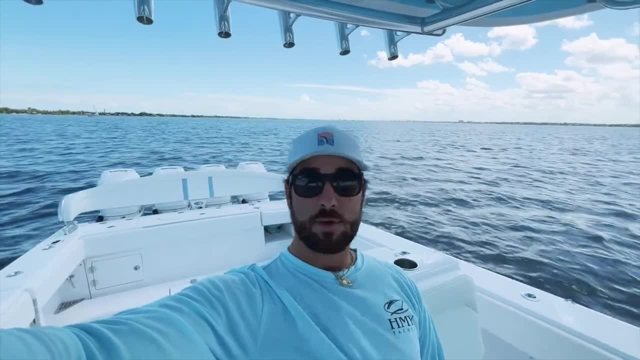 is staying in the state you're using it in. so that's that. let's go ahead and move on to safety regulations. these are things that you need to have on board your boat at all times. you need to have on board your boat at all times. you need to have on board your boat at all times. 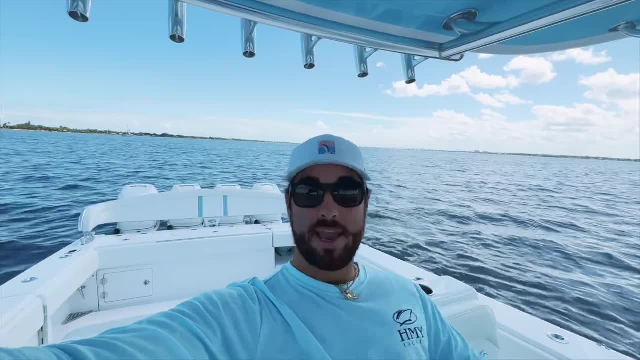 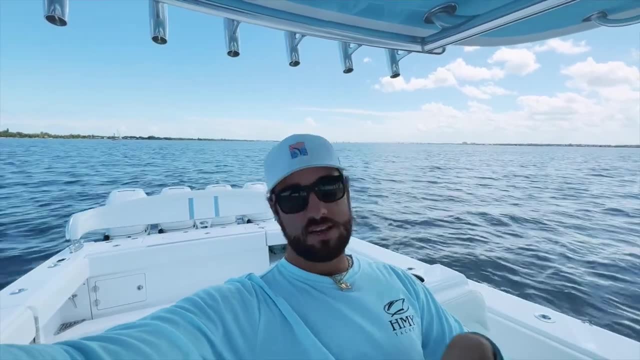 to legally be on the water. if you do not have one of these, you cannot be out on the water legally, and if you get pulled over, you can and will get a ticket and ask to go back to the dock. so let me actually pull the ones out i have on this boat and i'll walk you through everything. so the first and 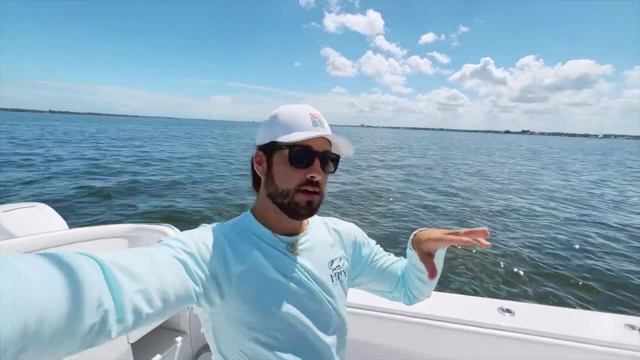 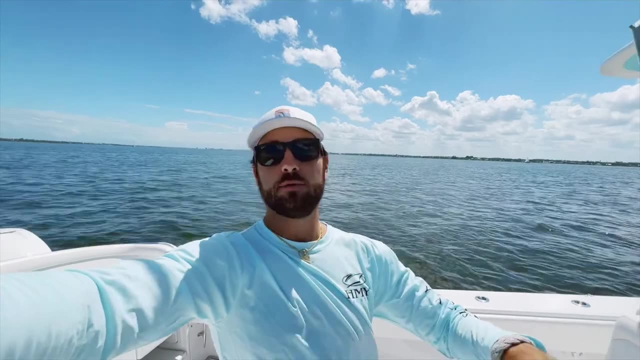 most important thing that you're going to need on your boat when it comes to safety gear is your life jackets- these bad boys right here, and for the regulations, you have to have one for every single person on board your boat at all times. if you have four people on board, you better have at least four. 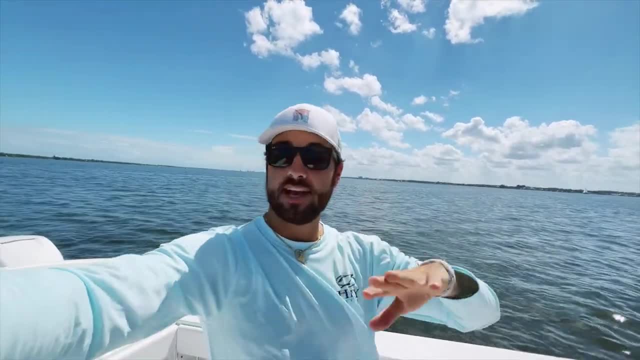 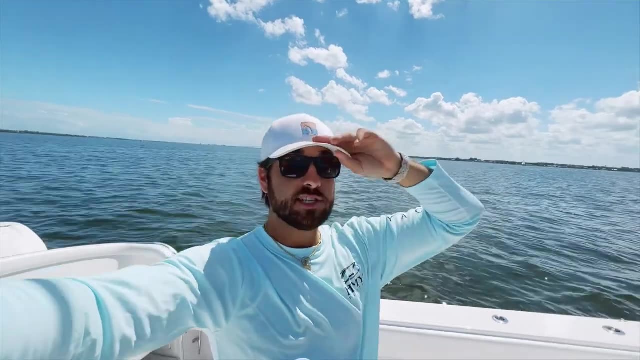 life jackets, or you can have one for every single person on board your boat at all times. you are breaking the law. if you have 10 people on board, have 10 life jackets. there are no exceptions to this rule. um, there are several different styles and kinds that meet the regulations. 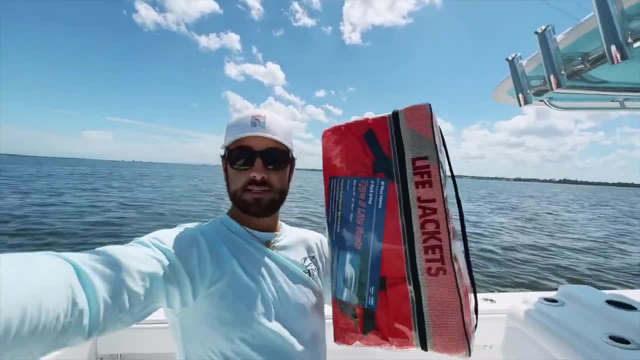 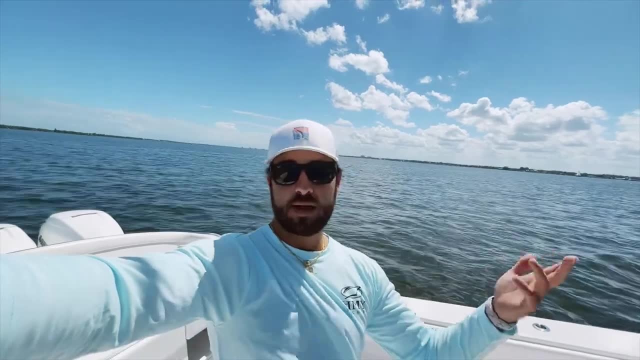 however, the easiest way to do it is take these. this is a pack of west marine type 2 pfts personal flotation devices. um, you can buy them at west marine. they come in packs of four. you know, if you're going to regularly have eight to ten people on your boat, go pick up three bags. 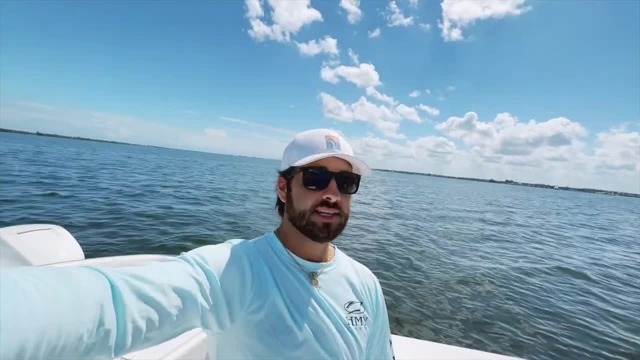 that's 12 life jackets- right there and store them somewhere where they're easily accessible and you're good. you never have to worry about it. you're going to be able to get them on board. you don't have to worry about it. i will always tell people error on the side of having way too. 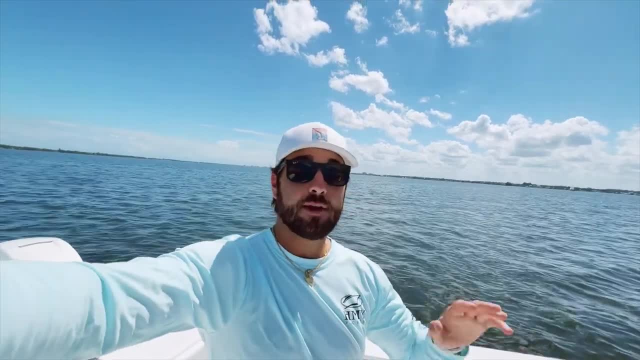 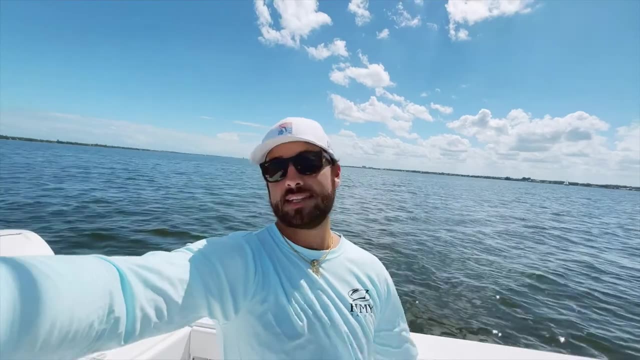 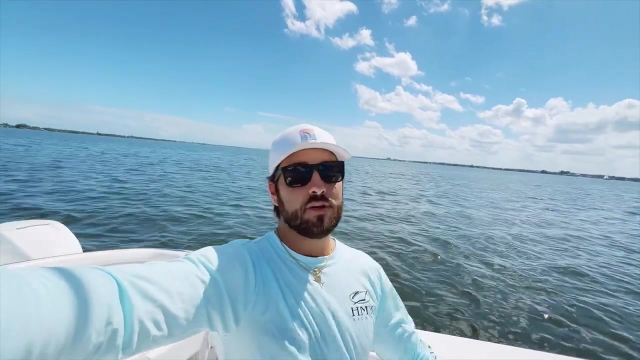 many life jackets on this boat. i keep 24 life jackets at all time. now, do i ever have 24 people? no, not really. i think the most i've ever had was like 16 to 20, and that was just sitting at a sandbar. i was not running, but you always want to err on the side of caution. you don't want to put yourself. 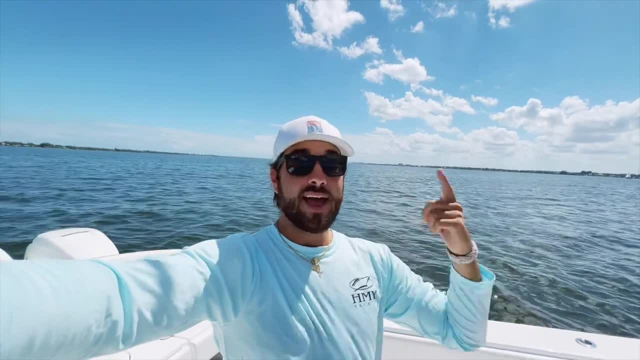 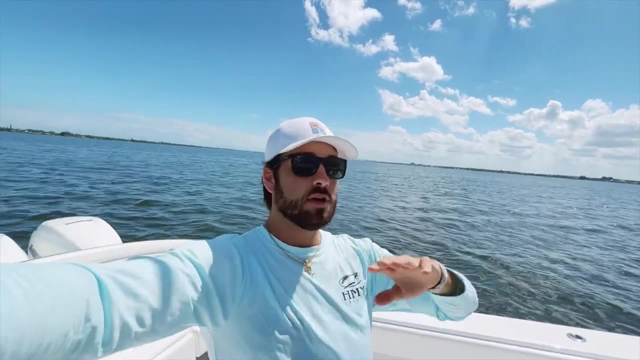 in a situation where you know worst case scenario that would actually sinks and not everyone has life jacket, but best case scenario: you just get pulled over. you don't have enough life jackets and you get a ticket. you want to avoid that? go buy your life jackets. have enough for everyone. 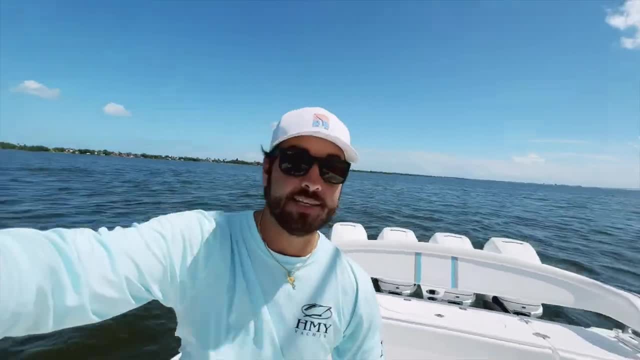 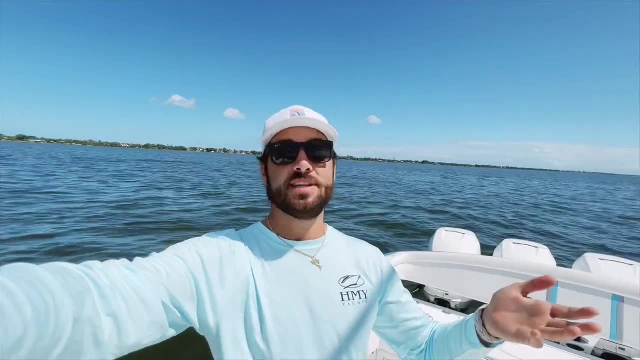 on board, and so the next thing that you have to have is this: a fire extinguisher, a certified fire extinguisher that has not expired. uh, fire on a boat is one of the most dangerous things that can happen for one. you don't really have anywhere to go jump on the water. it's not like you can. 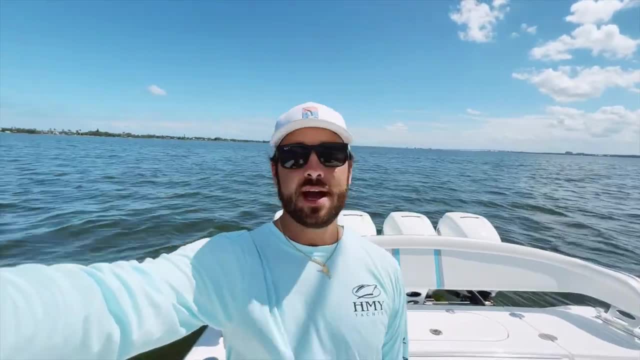 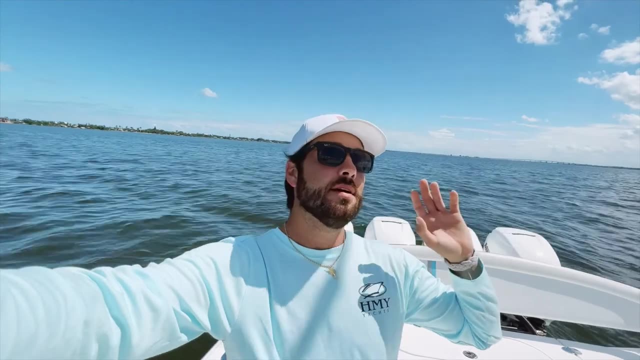 run away and you know, a boat is a thing floating out there full of a hundred plus gallons of fuel which, if that that catches it's just a big explosion waiting to happen. fires on boats are extremely dangerous. you need a fire extinguisher for one, for the regulations, but 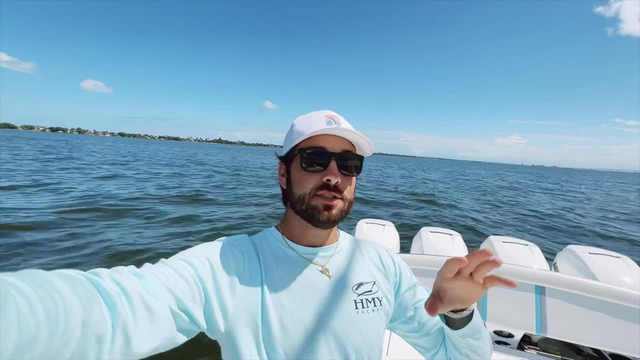 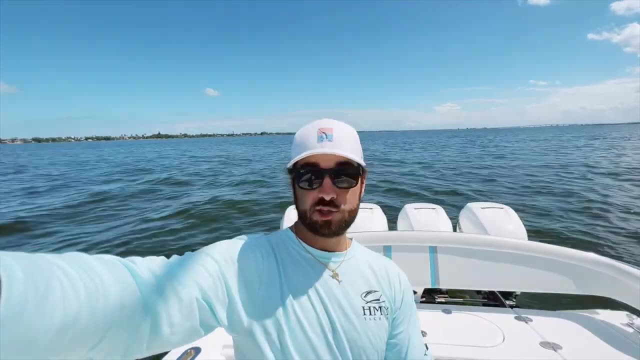 for two in the event of a fire. if you spend enough time on boats and complex boats with complex systems, you're gonna at one point run into somewhat of a scary situation. i've had it on this boat. i had a short in my undergun on life actually, luckily a fire did not happen. we caught. 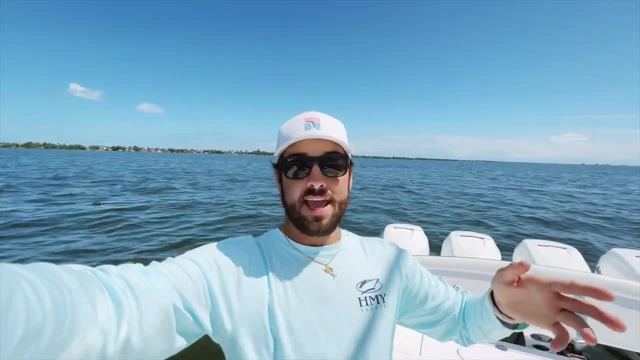 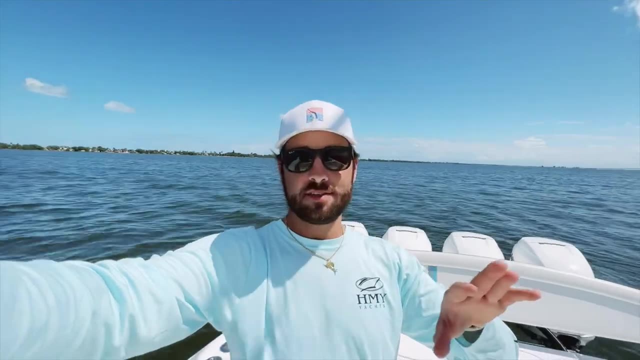 it. as you know, we just saw the smoke starting to come up, but that was scary because if that would have caught, we jump on the water and watch the boat go up in flames. so we're going to have a fire extinguisher. the next thing you are going to need is a sound making. 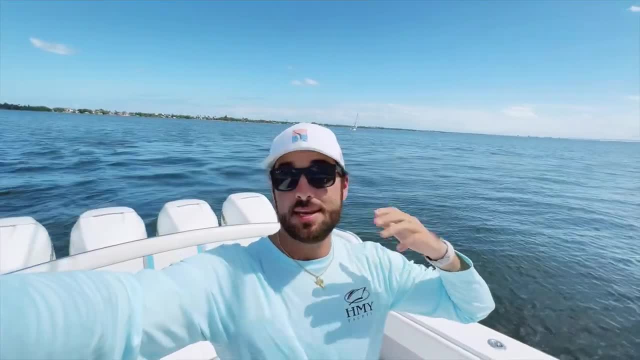 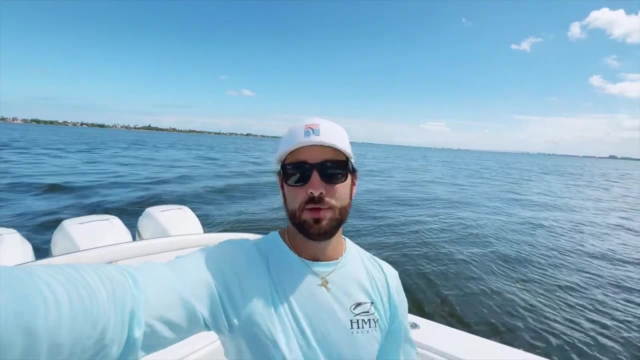 device, whether it be a whistle or an arrow horn, as long as it is an accepted sound making device. you can buy these little whistles, the ones without the balls, because those are not reliable. it looks kind of like a- i don't know- a usb drive almost, or you can get. there's all different shapes and sizes. 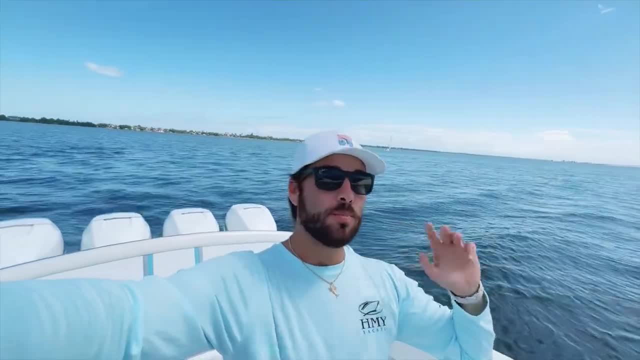 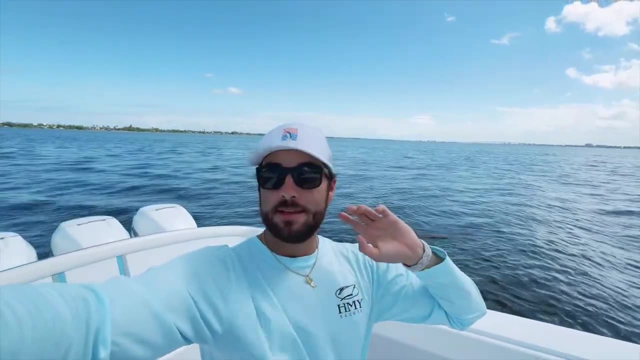 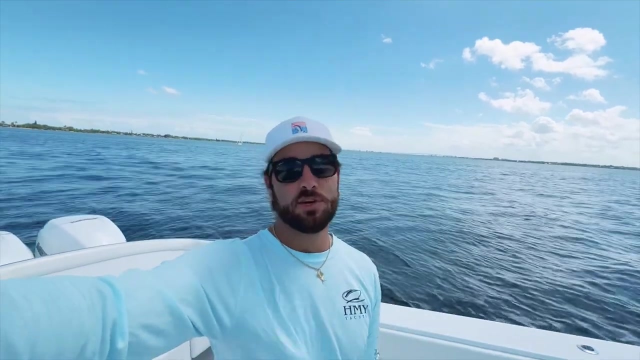 it's an orange whistle. it makes a loud sound. pick up one of those. or pick up a that is dangerous, very dangerous that. or an air horn- air horns, they suffice all the regulations. get one if you need it. you can press it loud noise. everyone around you knows what's going on. have a sound making device: the. 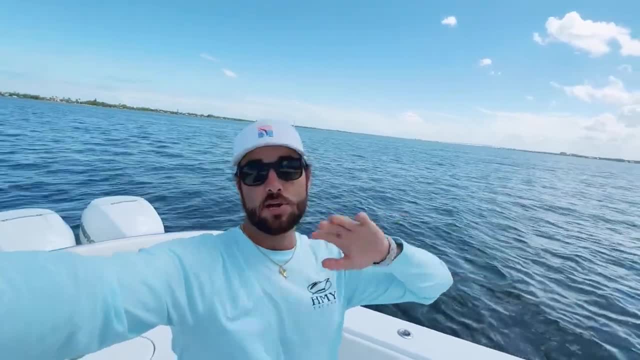 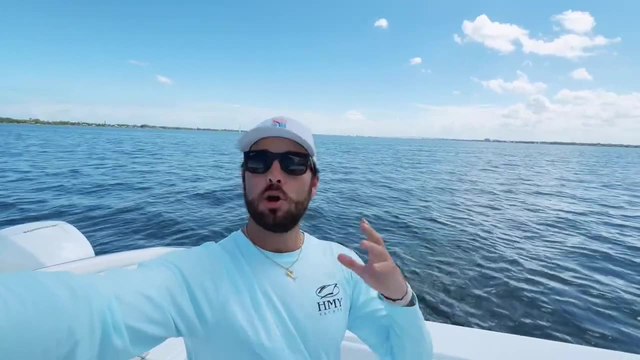 next thing you need is flares. you have to have a set of flares that are not expired, are current, and that's, you know, worst case scenario. you're out in the ocean, your boat sinking. you can shoot a flare up and hope that somebody in the area sees you, or it sinks, you're in a life jacket. 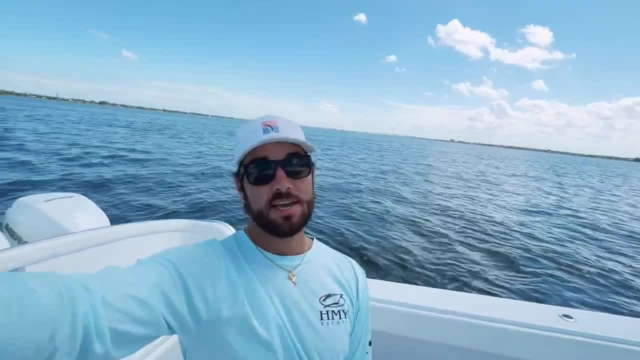 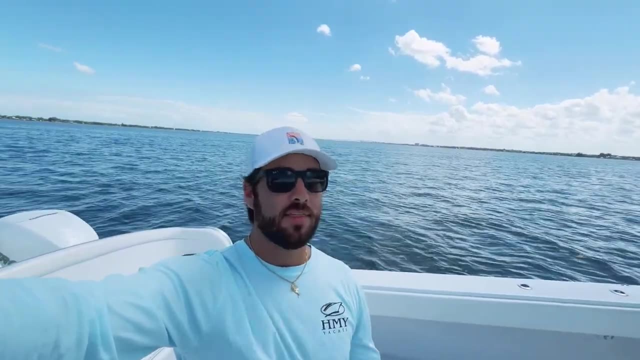 you're floating around, you have your ditch bag with you that has the flares on it, and you see a flare and you shoot up a flare. a flare is very hard to miss for anyone in the general vicinity, and so they'll see it and know that that's a distress signal and they will hopefully come to. 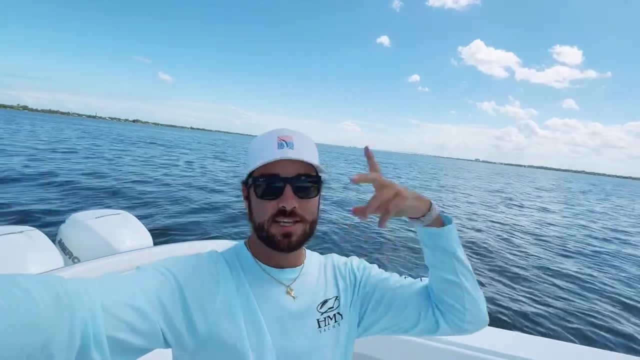 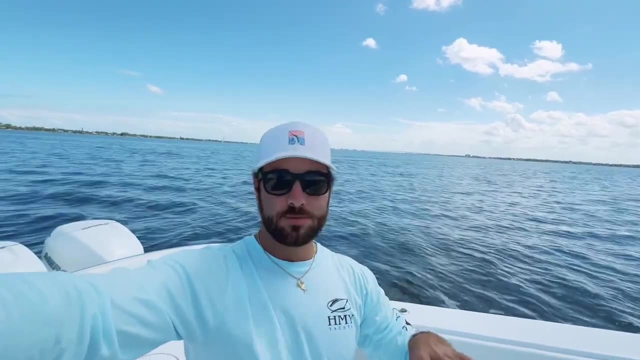 the rescue to save you. so you need unexpired flares. you can get stick flares, you can get the guns that you shoot up in the sky. there's a bunch of different times. just kinds just make sure you are getting approved non-expired flares for your boat. the next and last thing that you 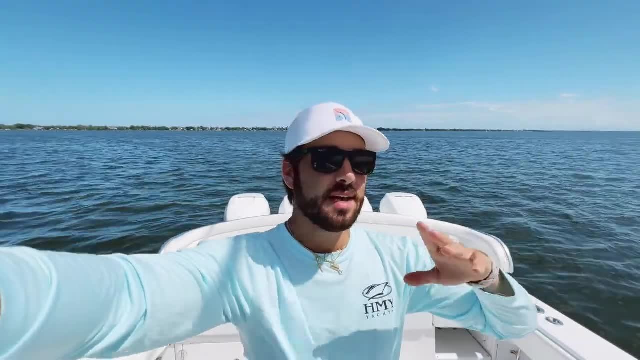 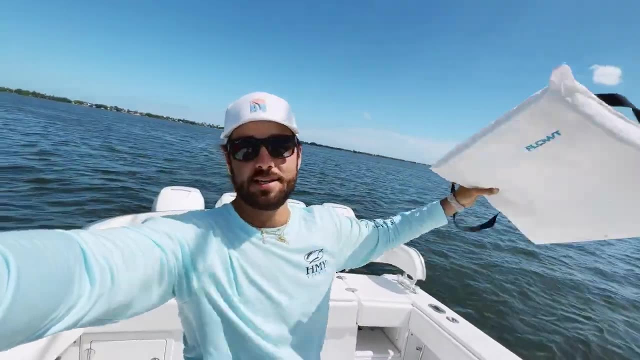 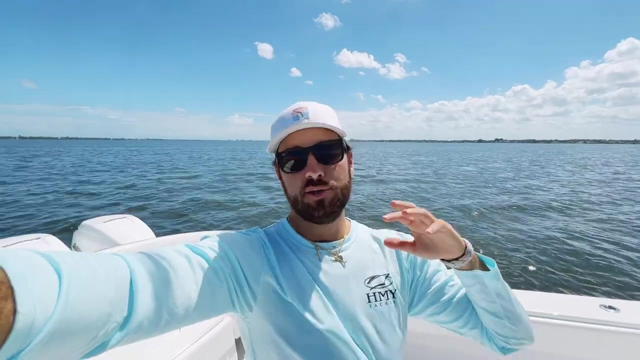 need is a type 4 throwable pfd personal flotation device. one you're going to see is this right here. it's just a square with handles on both sides, but that's for if someone falls overboard or whatever the case may be. you can throw that to them and they can grab it, hold on to it and use it as flotation. 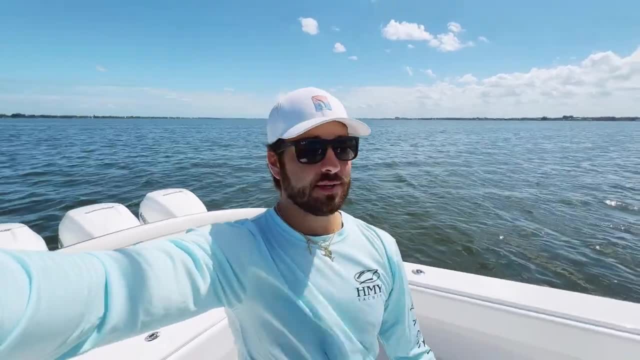 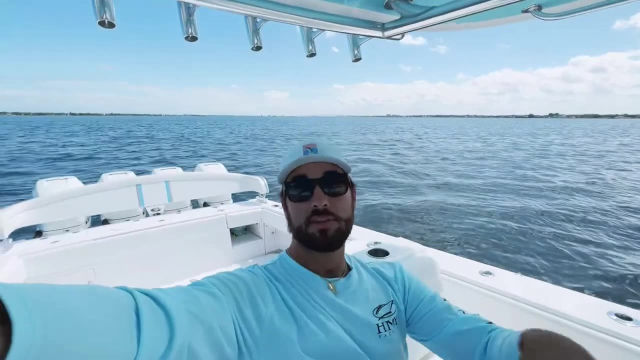 um, they're cheap, pick them up. we even keep two on this boat, just because you never know when you're gonna need to use maybe one for something else. cushion, whatever it is, have it on board. and one thing that i want to mention is that if you want to drive your boat at night time, which 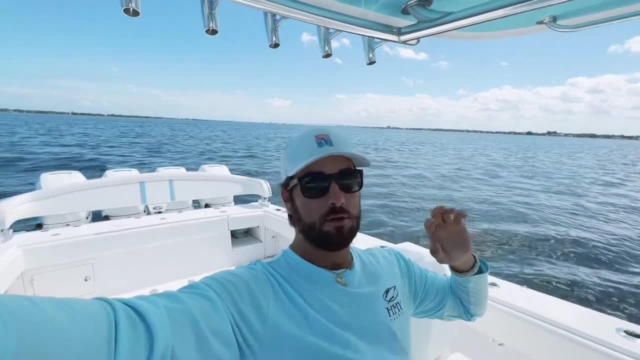 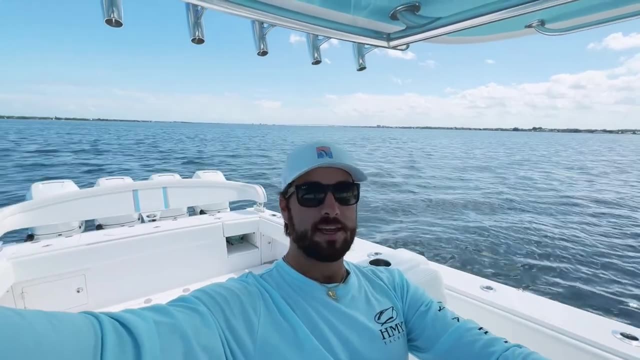 buys against. if you're a new boater, that takes a whole lot of skill, a whole lot of practice. don't do that until you are experienced. but if you're gonna do it, that requires a whole different set of you know things you have to have on the boat to run legally. in regards to 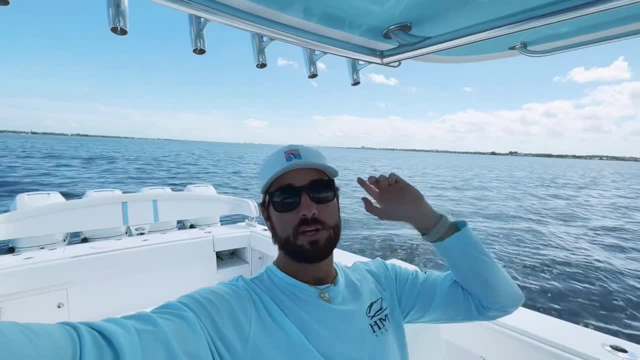 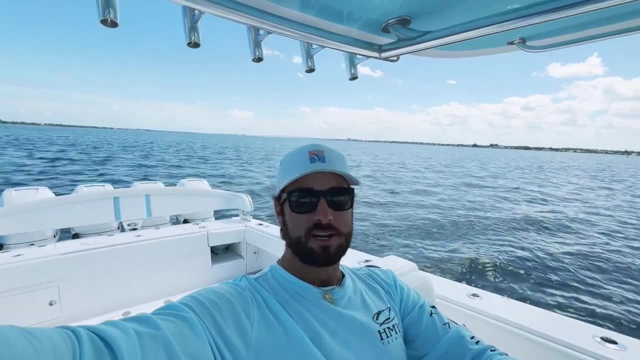 running lights- 360 lights. i made an entire video about that. i'm gonna go ahead and put that up in the upper right hand corner of this video. watch that video if you're interested to see what you need. if you want to run a night time, let's go ahead and move on to the rules of the road now. 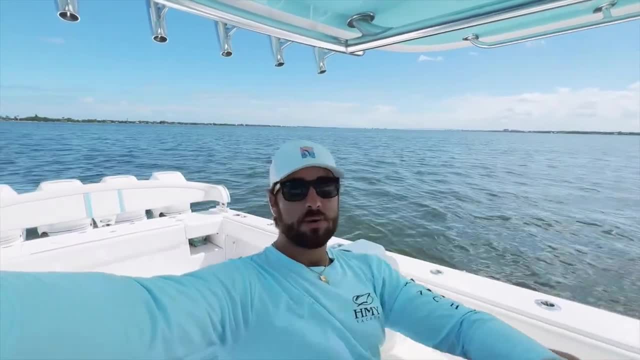 so next we're going to attack the rules of the route. now here's a couple of things that i want to talk about. first, the rules of the road, The rules of driving a boat in the water and how you need to act around other boats, And this is a very long-winded subject. I could make an entire three-hour. 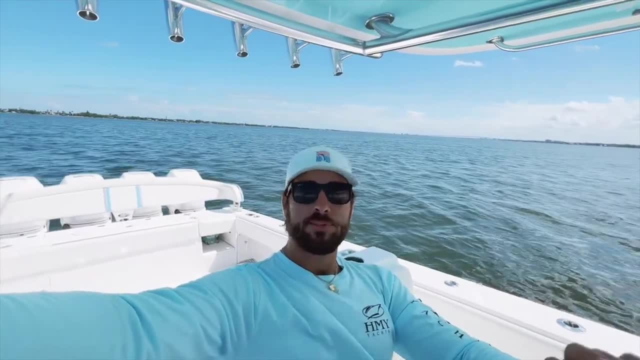 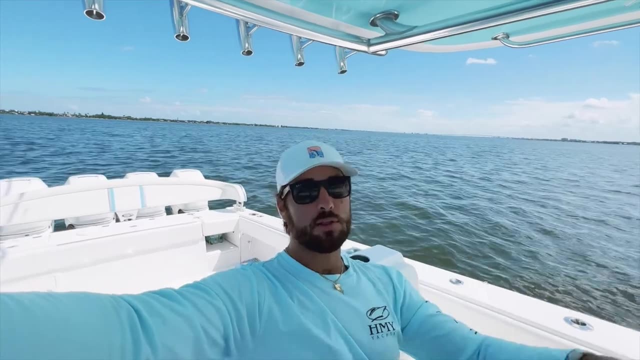 video on this and still not touch half of it. So I think the best way to attack this one is to just touch on the very basics that somebody needs to know to go out on the water and be safe and not be a hindrance to other boaters. Things like how to pass a boat if you're coming up behind somebody. 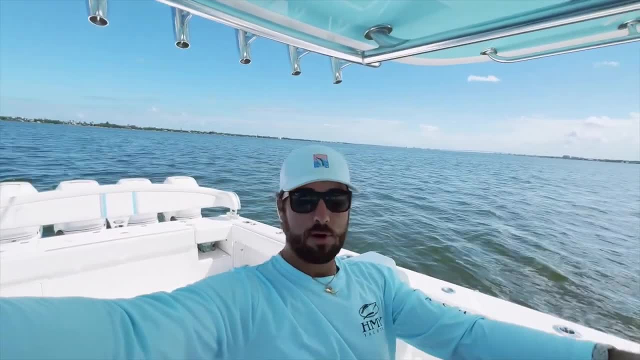 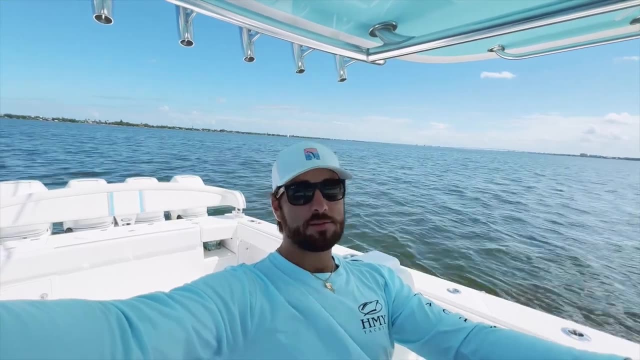 how to pass a boat if you're approaching head-on, how to read channel markers, all that kind of thing. And I think the thing that makes the most sense to start with is passing boats Because, realistically, once you're out in open deep water channel markers for most recreational boats aren't. 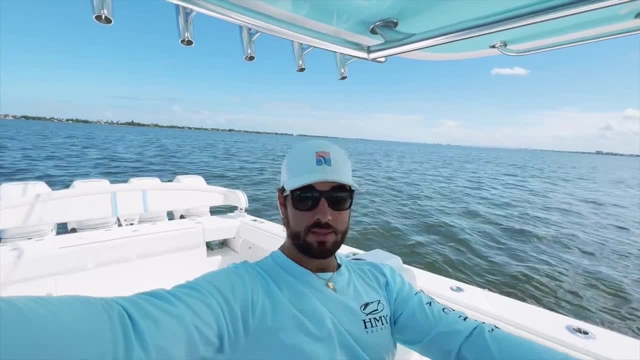 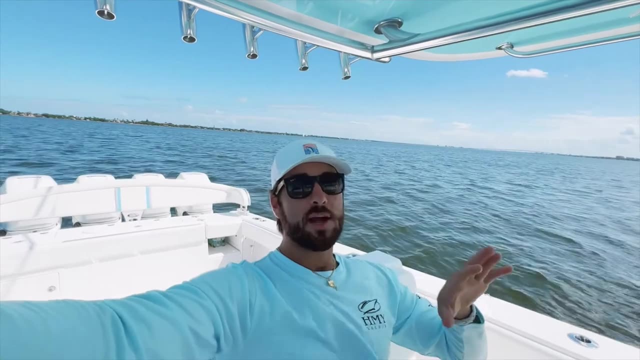 crazy important, But passing boats is extremely important. If you pass incorrectly it can be dangerous for everyone. You can cause a collision the whole nine yards, And so let's go ahead and start with. if you're passing a boat head-on, You know you're heading north. there's a boat heading. 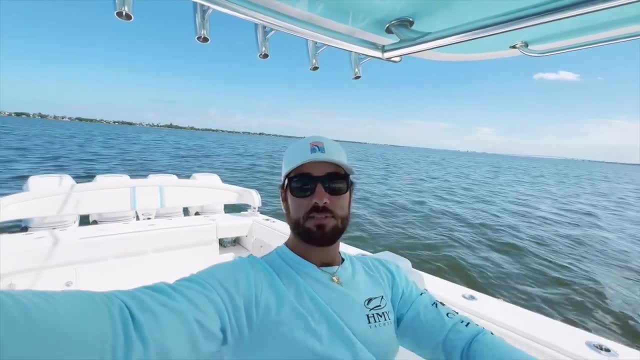 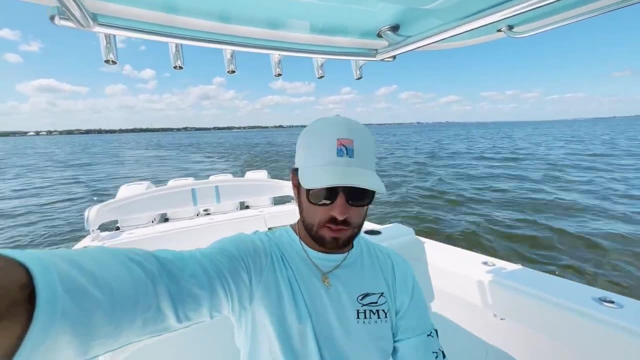 south straight at you. How do you pass a boat head-on? You're passing a boat head-on. you're heading south straight at you. How do you deal with those situations? So you're heading down a waterway, there's a boat heading towards you. What do you do and how do you safely pass it? And so, 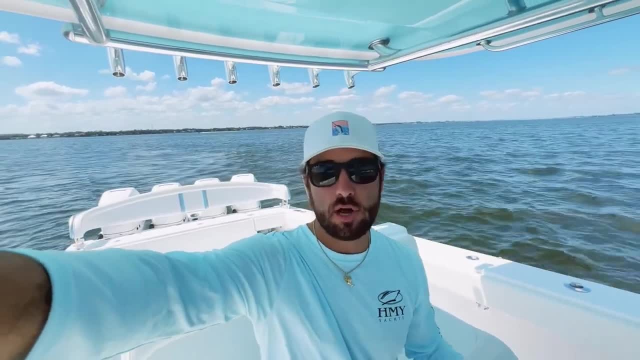 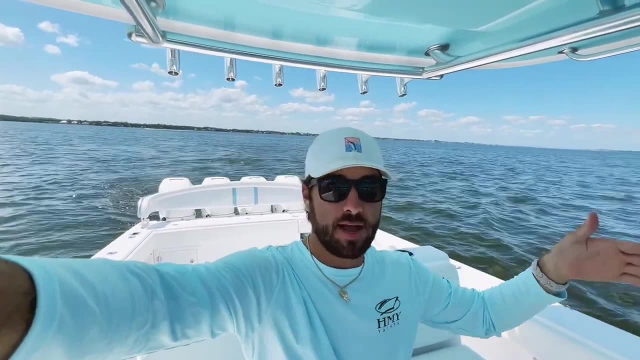 it's pretty simple and it's quite shocking that a bunch of people just don't know this. But basically you want to pass with the boat on the port side of your boat, The port is the left side when you're facing the bow, The starboard is the right side when you're facing the bow, And I'm going to kind. 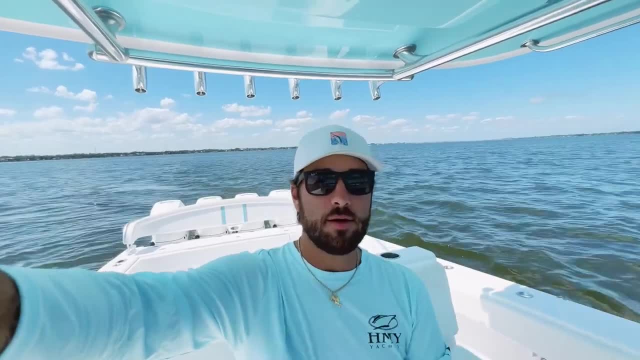 of demonstrate this right now. I'm currently going down the waterway. There's a sailboat out there. I don't know if you can see it. I don't know if you can see it. I don't know if you can see it. 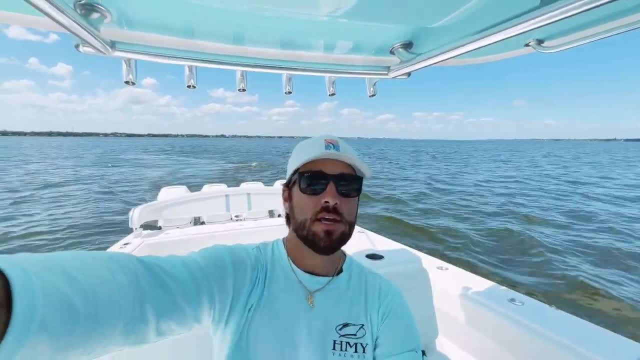 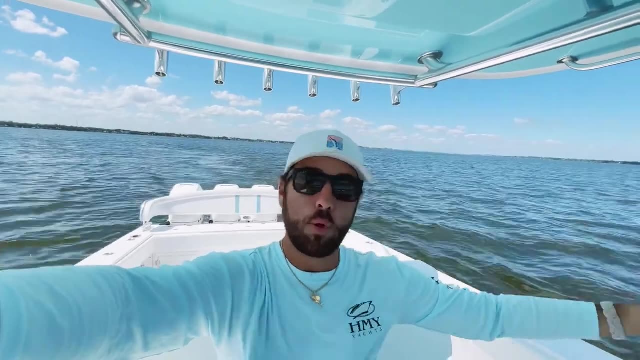 But I'm heading towards him, He's heading towards me. You're going to want to alter your course a little bit to the starboard, to the right, so that that boat can pass safely off of your port side. And that boat, if they know what they're doing, should do the same thing. They should alter their. 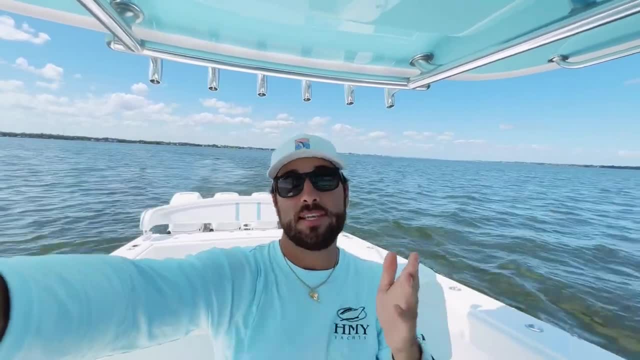 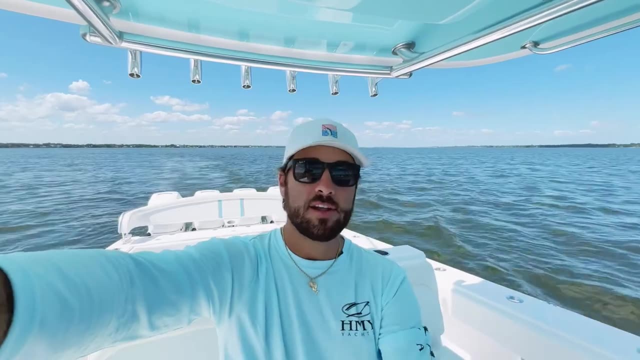 course, alter their course a little bit to their starboard. you know, take a slight right turn to make sure that you guys pass along each other's port side without any interference. You can see I'm here, The boat is up there. I'm going to take a. 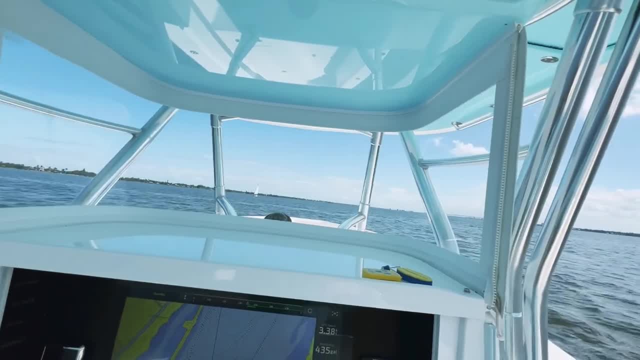 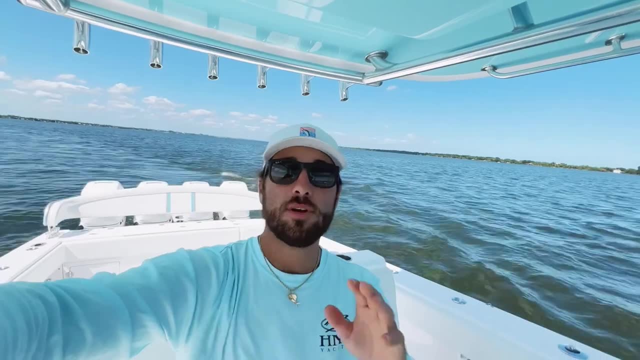 little right turn which puts me passing off the port side. They're doing the same thing. We're no longer in harm's way And those are the rules of the road And everybody needs to abide by that, Because if you have a boat behind you or there's a boat behind that boat and you 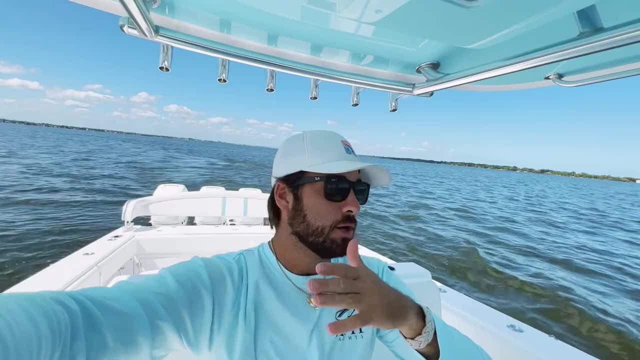 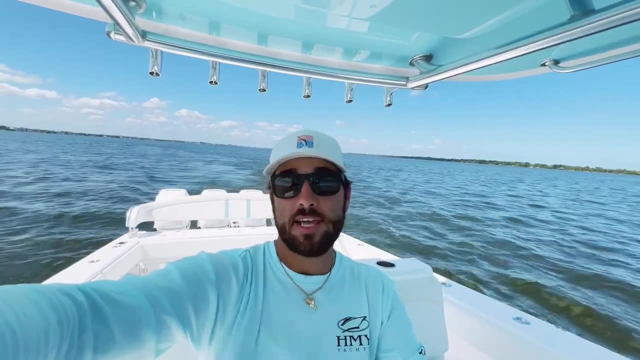 don't know what you're doing. and then that boat doesn't know what you're doing And so if you go to the left and try to pass them, so they say to your starboard side, you know they're going to. in their mind they're going to go, take a right turn, you know, to try to keep you on the port. 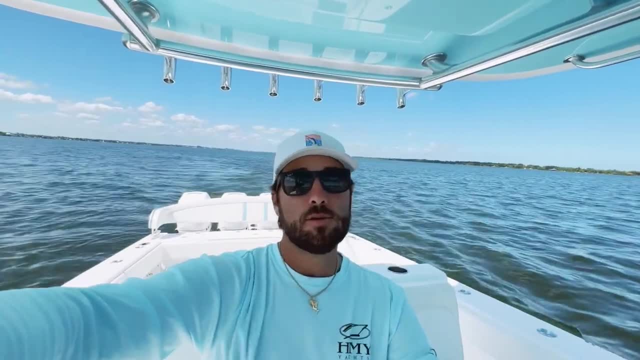 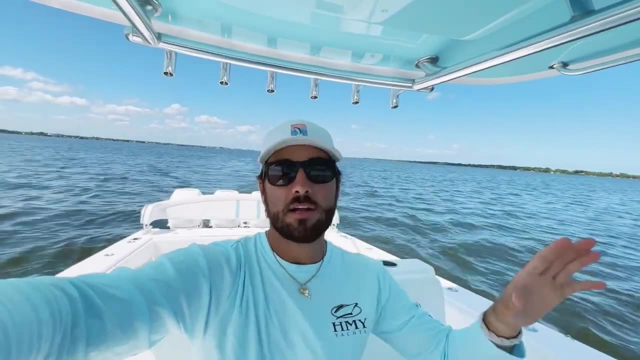 side, but you're taking a left turn to keep them on your starboard side. You both are turning straight into each other at the same time. You're both going to have to slow down, come off plane the whole nine yards And it just is not good for anyone. You need to know how to pass people. 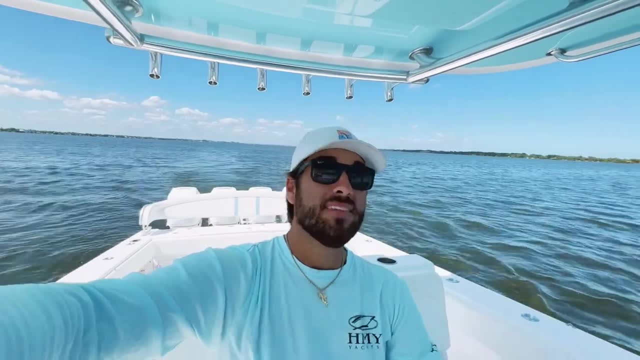 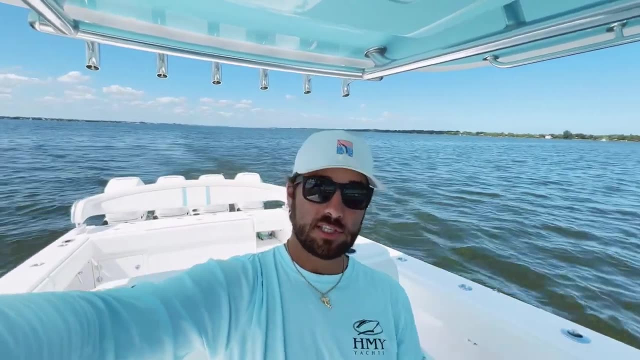 keep them off of your port side at all times, And that goes the same when you're passing somebody from behind to you know, someone ahead is ahead of you and they're going a little bit slower than you and you want to pass them Legally. you never want to take a left and go around. 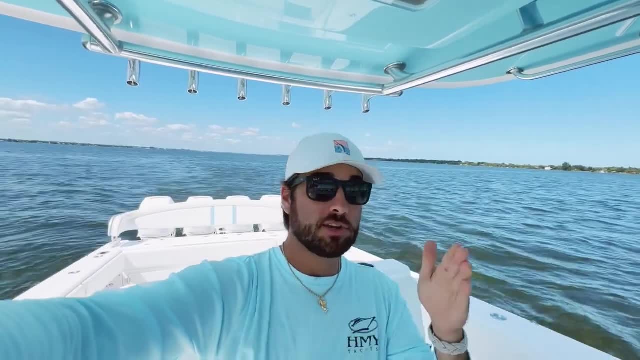 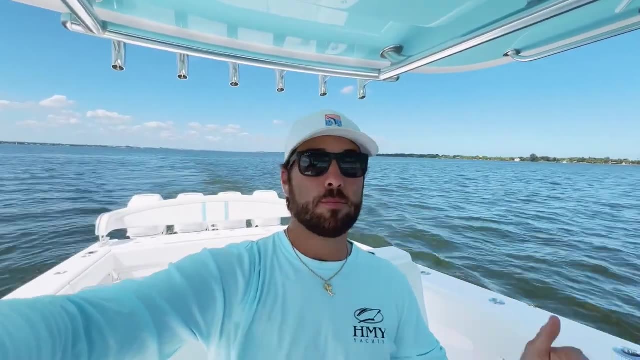 They're port side. You want to take a right and go around their starboard side, keeping them off of your port side. Anytime you pass a vessel it stays off of the port side of your boat And that boat that is being passed needs to. you know the captain needs to have his head on a. 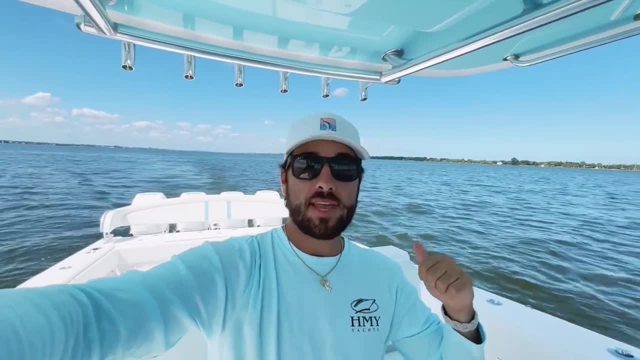 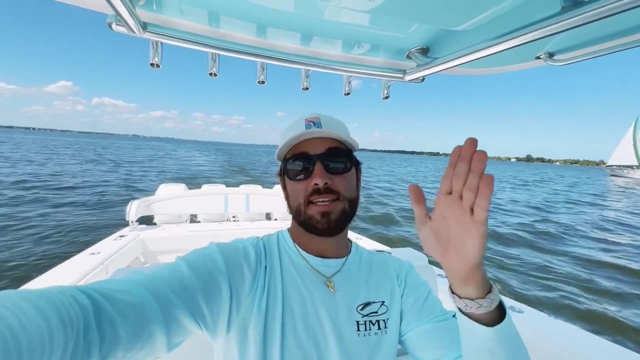 swivel and needs to know what's going on. He needs to know that there is a boat that is coming up behind him And his job is to keep his course, his same course and his same speed and not alter from the boat. And so if you're the boat that's being passed, you're going slow. someone's coming up. 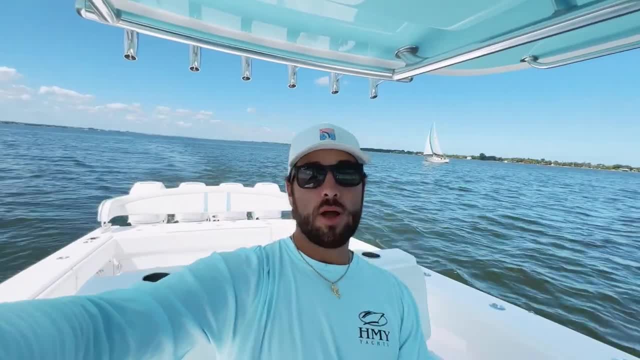 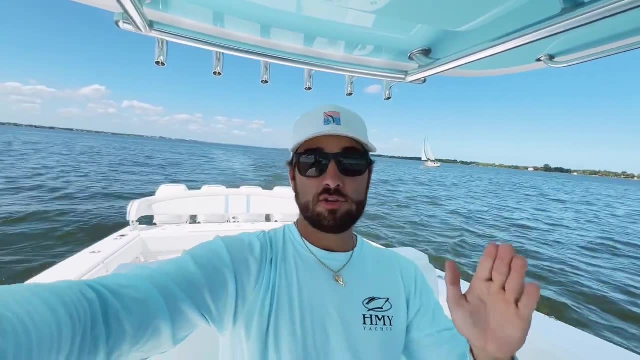 You need to know that there's someone behind you. You should be looking around at all times to know what everybody is doing around you and what's going on. And if you see a boat coming behind you who's getting ready to pass you, do not change your course. stay your same course. stay your. 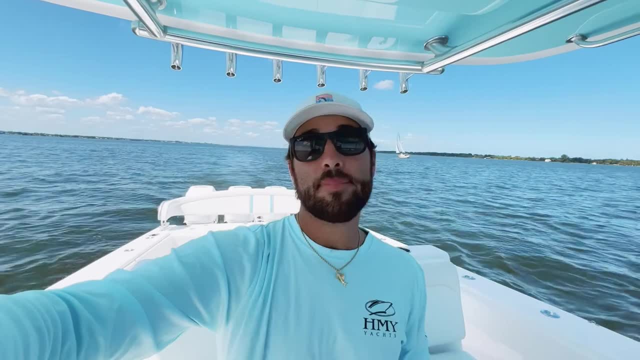 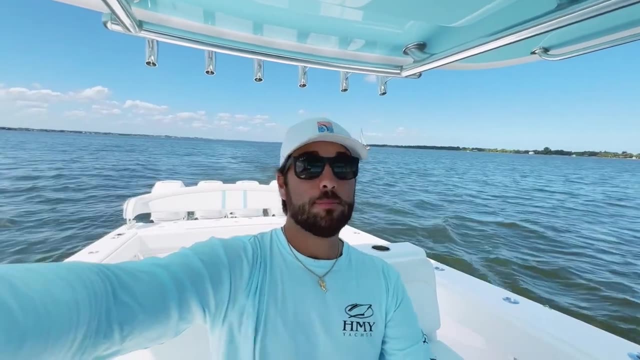 same speed. That is your responsibility as a boater. If something happens and there's an accident and you have to go to court for it, they're going to assess the details and you will be at fault. If you did not, partly at fault. 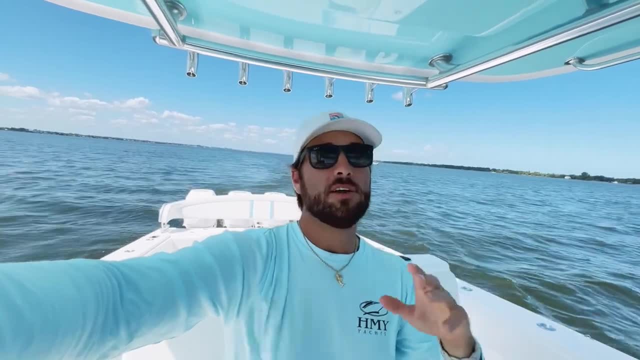 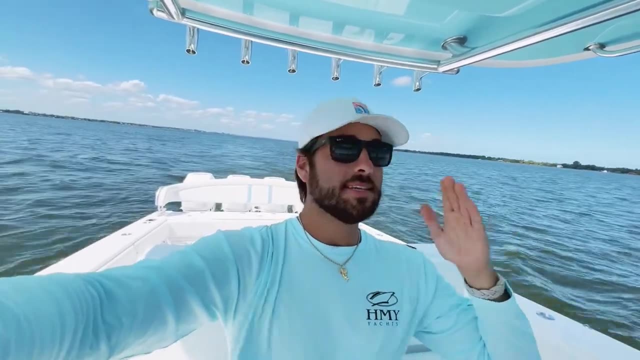 If you did not keep your course and speed, that is on you. To know what's going on around you, to know there's a boat coming up behind you to pass, you keep your speed And if that's if you're the boat doing the passing, keep them off your port side. So I know that was. 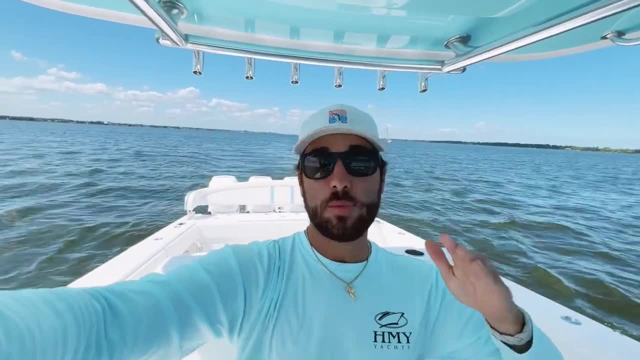 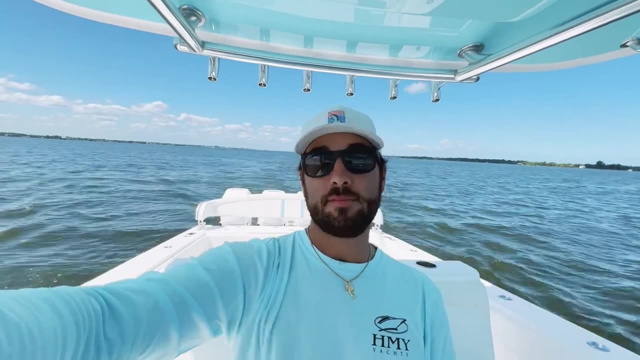 long-winded. but a quick summary is always, if you're doing a passing maneuver, keep the other boats to your port side. If a boat's coming head on, take a slight right turn. They should do the exact same thing from their point of view And you guys will pass port to port If you're coming up. 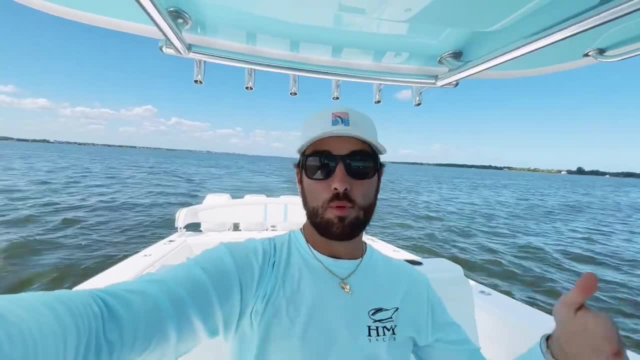 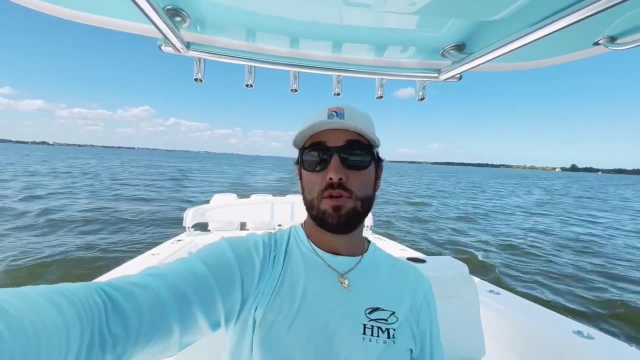 behind the boat, take a right turn and pass So they're on your port side. If you're the one being overtaken, know that there's a boat coming behind you and stick to your same course and speed so that you don't create any confusion or any problems or anything. So, obviously, every passing situation 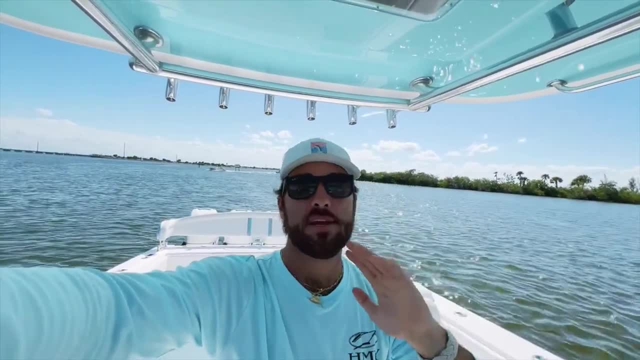 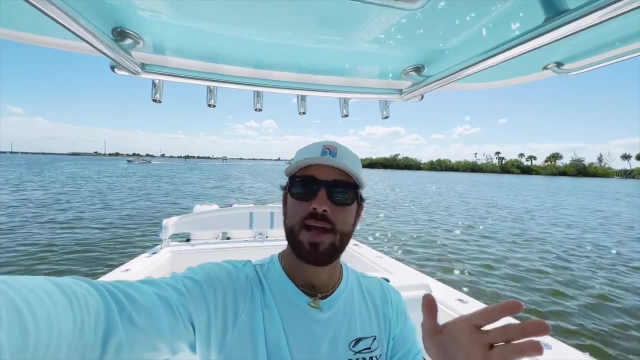 is not going to be when a boat is coming from behind you or straight on. you know boats are everywhere coming and going in every general direction And it's pretty straightforward in those situations Your boat can kind of be divided up into four quarters. You have your starboard bow as one quarter. 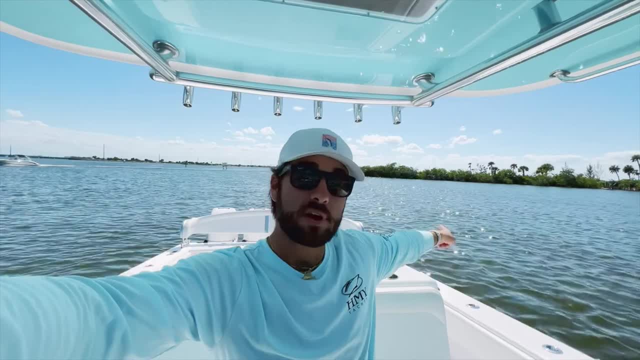 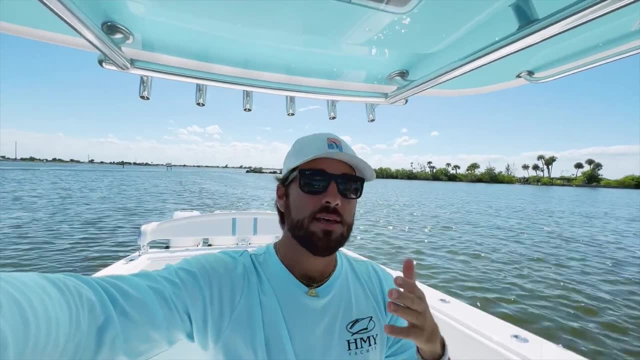 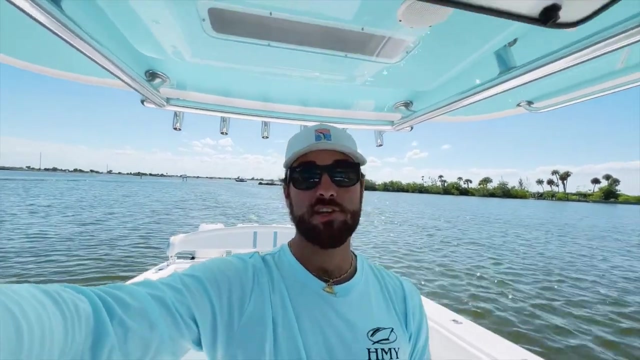 your starboard aft section is in one quarter, your port aft section is another quarter and your port bow as another quarter, And so basically, your starboard bow quarter any boat that is in that corner in your line of sight. you know, from the bow to the right. 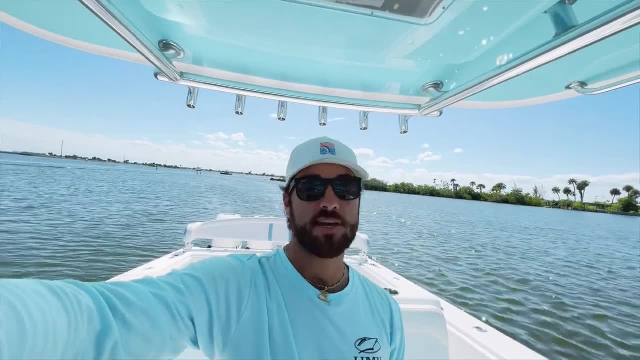 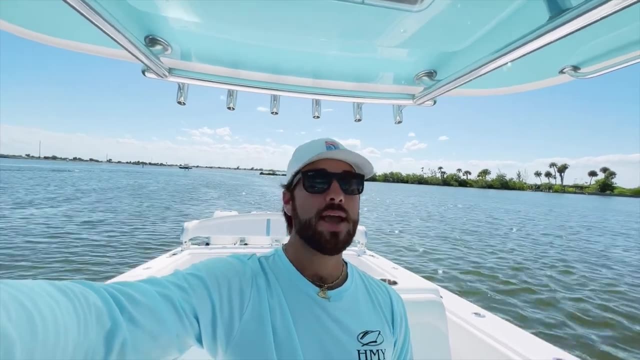 and midship forward. you have to give way to that vessel. if you're in a crossing path, You slow down or you take a right and go around behind them, And then you have to give way to the other boat that's in that corner. 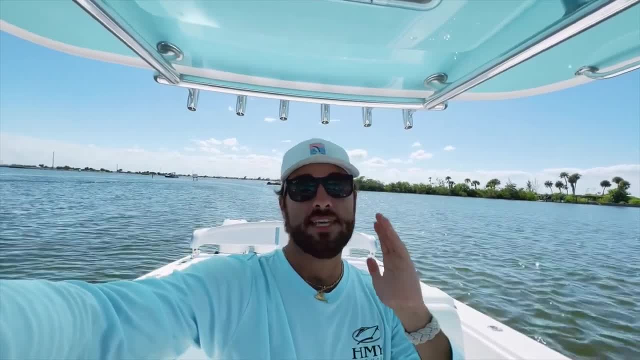 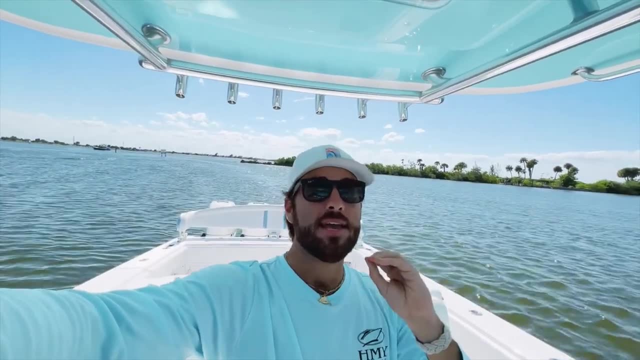 So if you're in a crossing path and you have a boat in any other quarter, you know any boat to the left of your bow, any boat behind you, anything. you have the right to keep your course and speed and they have the responsibility to go around you. 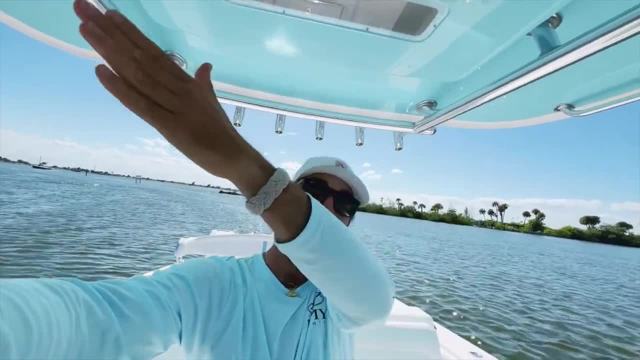 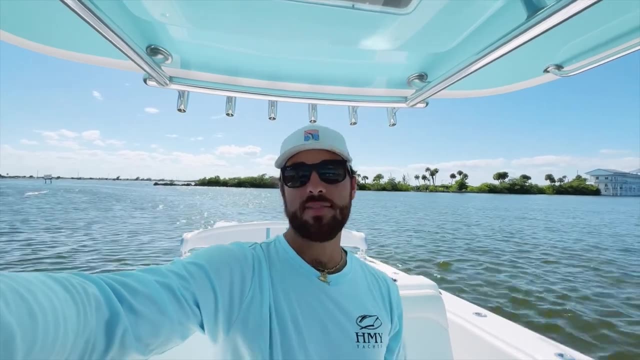 The only time you really have to give way is if there's a boat that's to the right of your bow, forward of your midship line. you know, in that first quarter over there It's pretty straightforward rule. If you know the boats around you, you know keep an eye on that. 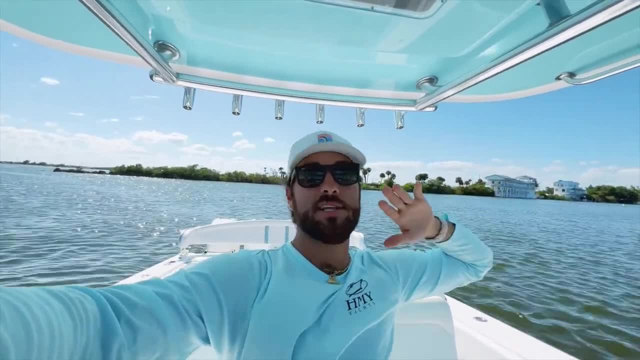 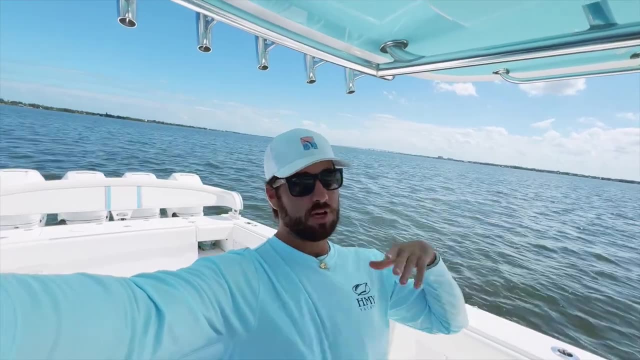 If you're in a harbor bow quarter, they should take evasive action and get around you as long as you are keeping your course and speed. And one thing that I must mention is that if you're going to be fully legal and fully compliant with the rules is if you're overtaking a boat from behind. 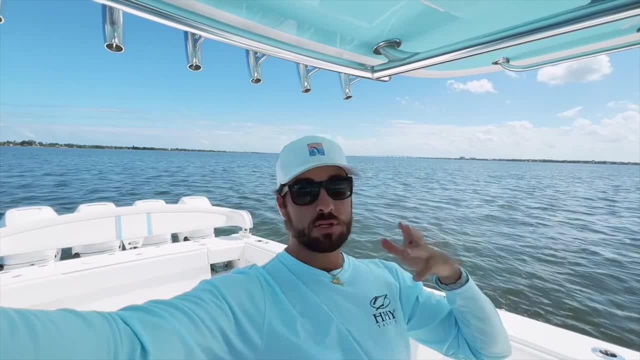 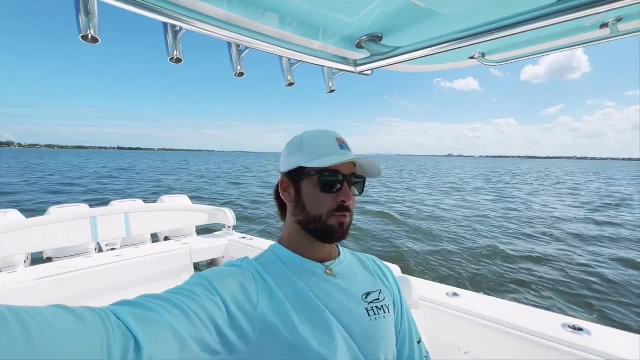 there is a horn, a sound that you're supposed to make. I forget if it's one or two horns, whatever it is, or one long blast, But I know, realistically, most people are not going to do that. Most people don't do that. You know, in the recreational world I don't see anyone do that. 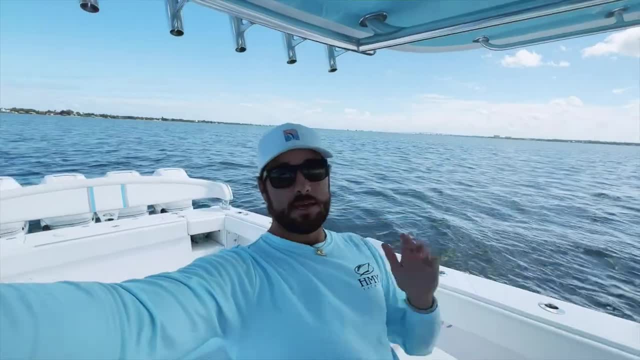 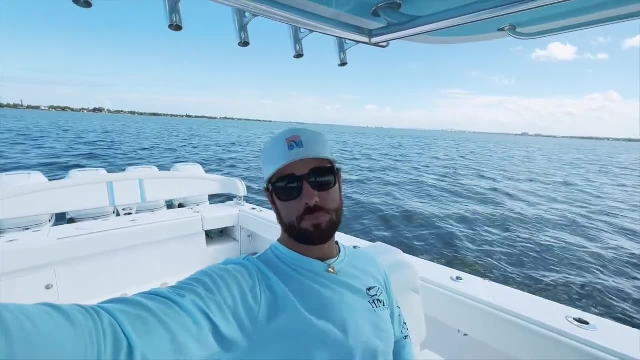 So it's not realistic Head on a swivel and know what is going on. And something else that I do need to mention is that the very first rule in the rules of the road is that you, as the captain of that boat, you have the responsibility to avoid a collision at all costs, even if that means breaking some. 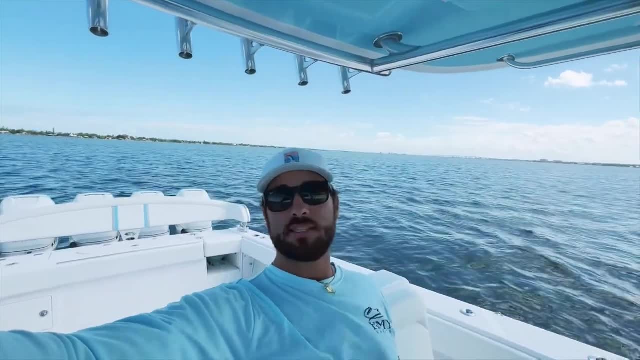 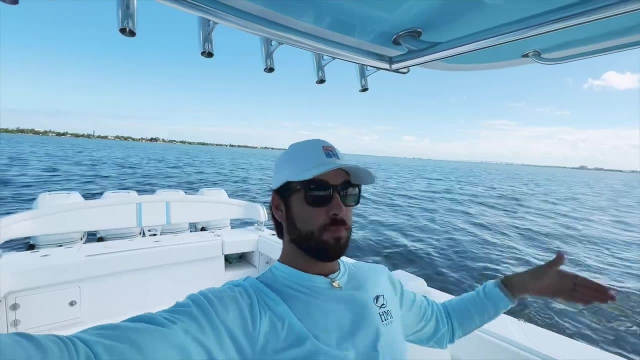 of the following rules about passing a boat. You know if you're coming up behind somebody who's going slow and you need to pass them, but doing so by taking a slight turn to the right starboard to keep that boat off your port side is going to cause a collision or is going to be dangerous. 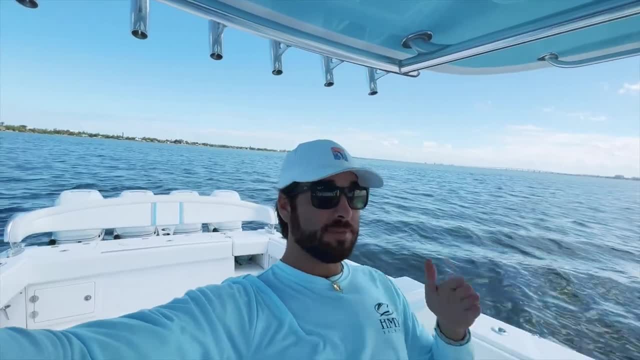 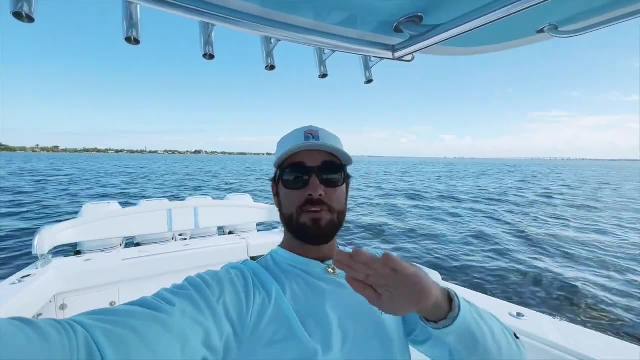 for any of the parties. Do not do that. If you, as the captain, deem it is safer to do so by going around the port side of that vessel and keeping them to your starboard side, you have the authority to do that. If at 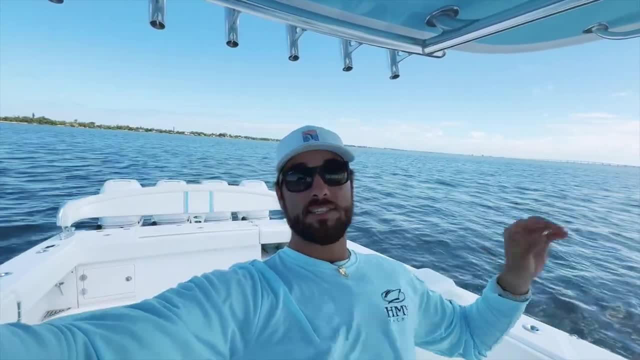 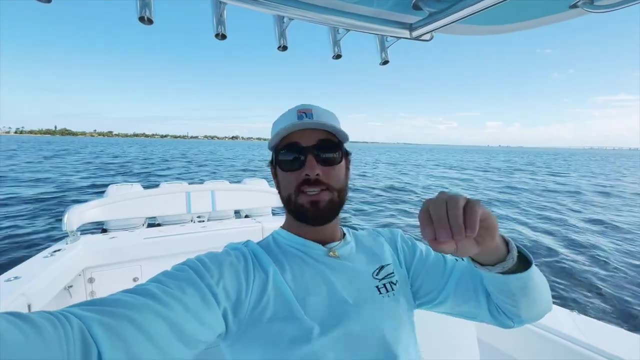 all possible, you need to try to keep them off your port side. But if that's not safe and the only safe way is to go around the other side, you do have the legal authority to do that. You need to avoid a collision at all costs If anything happens and you again something happens. 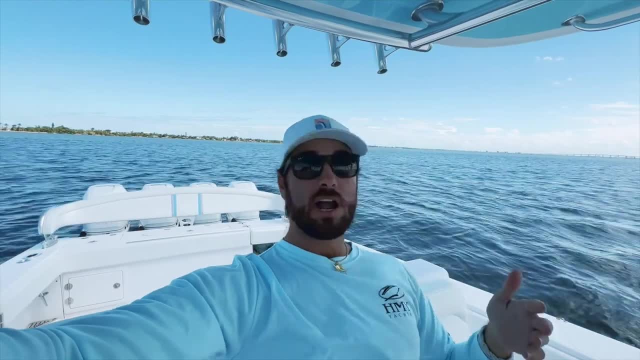 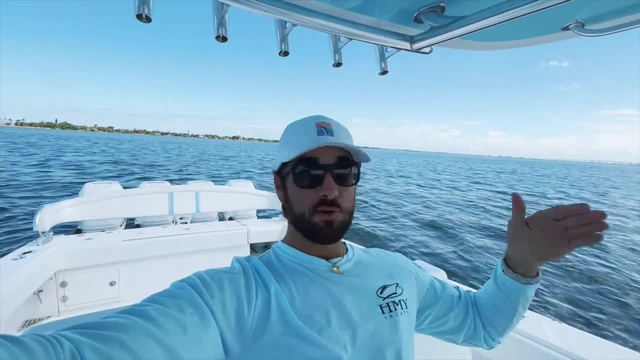 a collision happens and you have to go to court And you cannot prove that you did every possible thing to avoid that collision, You will be partly at fault, even if it wasn't mostly your fault. So that is something that must be noted. 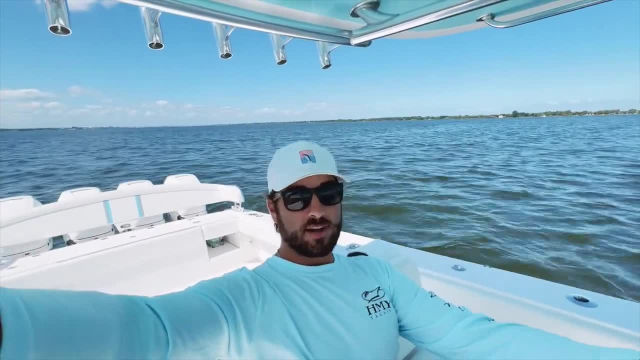 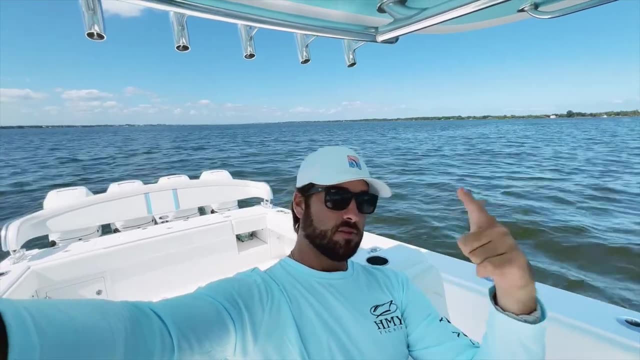 And so something that I forgot to mention was there is a hierarchy of the different kinds of boats, and who has to give way to who you know, whether it be sailboats, cargo ships, fishing vessels actively involved in fishing or trawling. 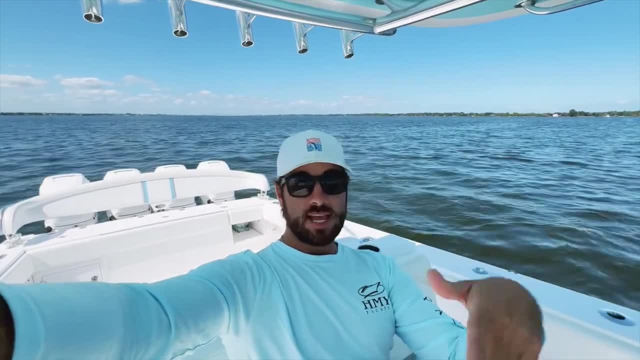 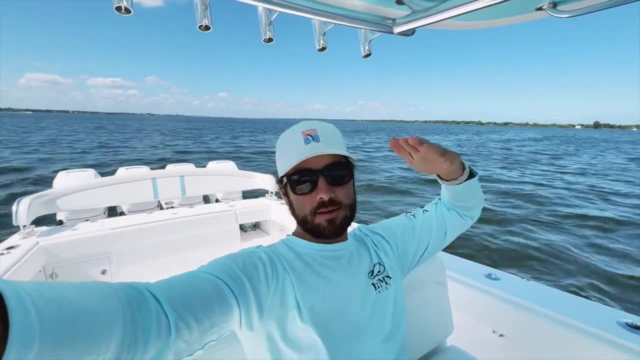 vessels restricted in their ability to maneuver due to depth, whatever it might be, You know there are. you know, like for a powerboat, we have to give way to sailboats, to cargo boats, anything else, For the most part, anyone watching this video is going to. 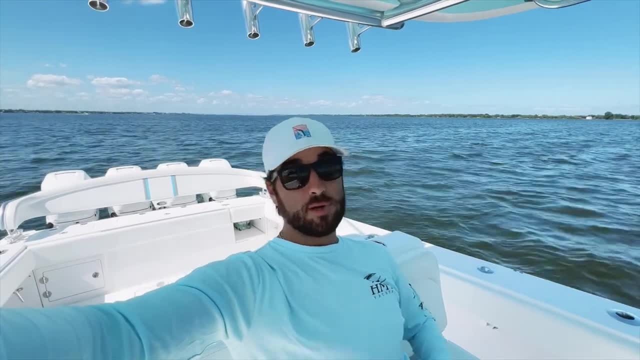 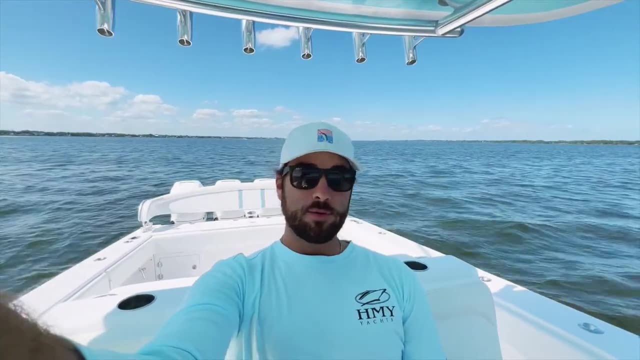 be in a powerboat with an outboard or an inboard, which is a very maneuverable boat, And so, realistically, we have to give way to everybody If you come in a situation where you're, you know, around sailboats that are sailing, fishing vessels, cargo ships, whatever. it is general. 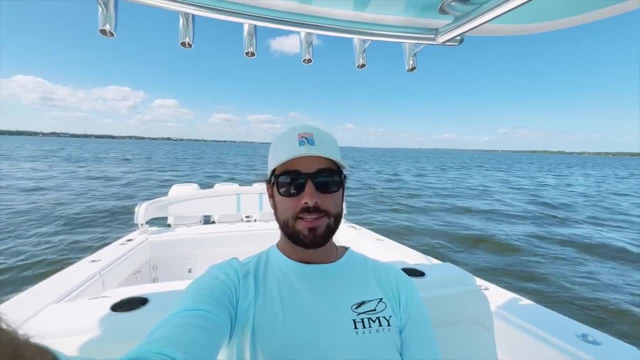 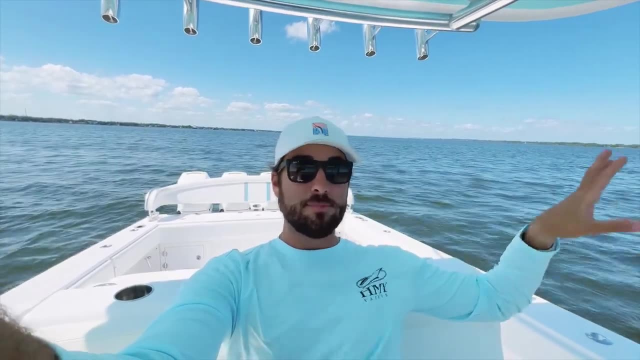 thumb. stay away. let them do what they want to do and do not get in their way. We are the most maneuverable boats on the water, and so because of that we have the responsibility to get out of less maneuverable boats away. There's a lot more to it, but if you abide by that rule, 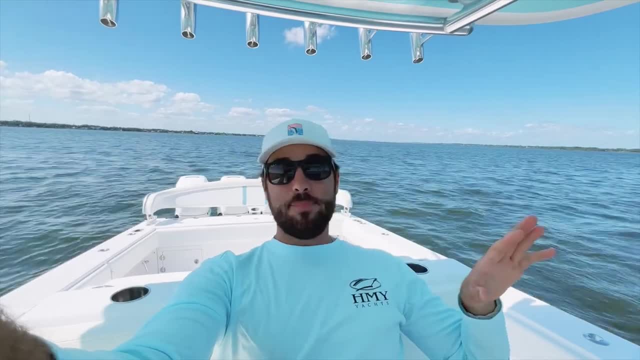 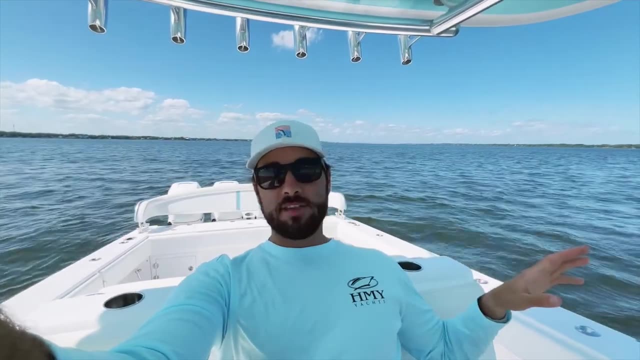 you'll never have a problem. Basically give way to any bigger boats, commercial boats, whatever it is. let them do what they want to do and steer clear You're. you're in a maneuverable boat. you're not actively involved in any commercial operation. get out of their way. 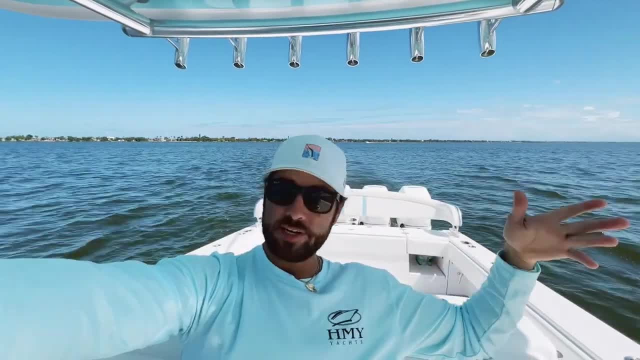 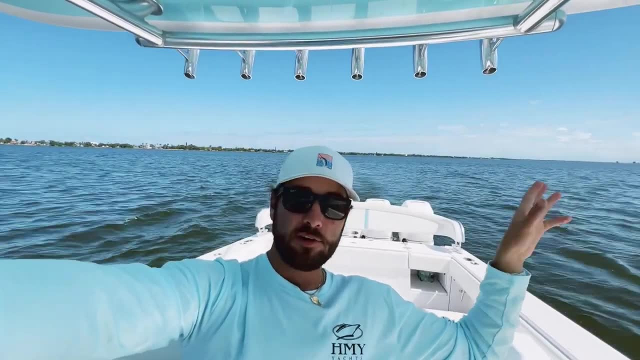 So the next topic that we're going to tackle is channel markers, and these are pretty simple, Chris B. There's really not a whole lot of nuance to it. You know you're going to see, at the very base level, two types of channel markers: red ones. 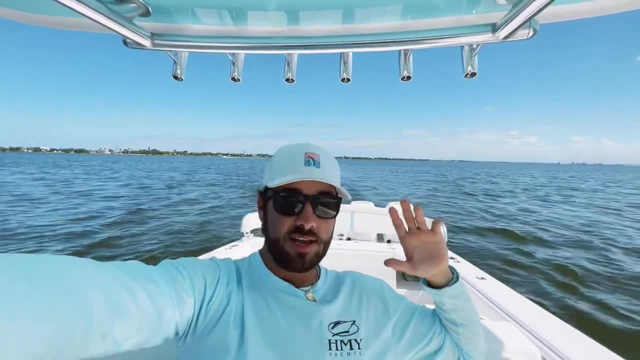 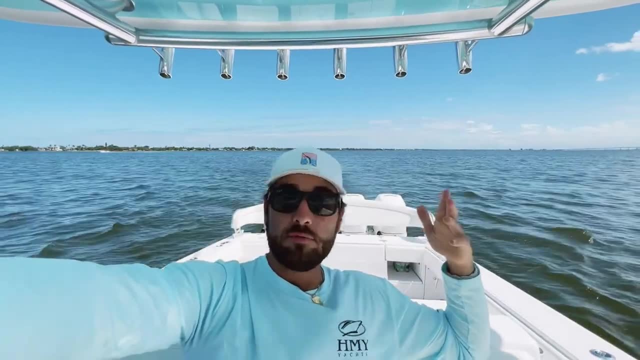 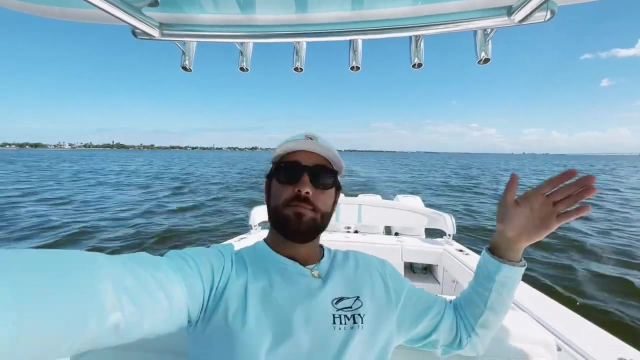 and green ones When you're coming in and out of a marina, in and out of a port, if you're coming in from the ocean through an inlet. the general rule of thumb- well, not the general- the rule of thumb is to keep the red markers off of the starboard side of your boat at all times. There's 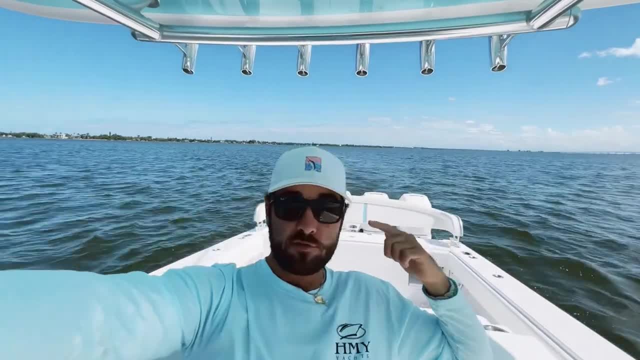 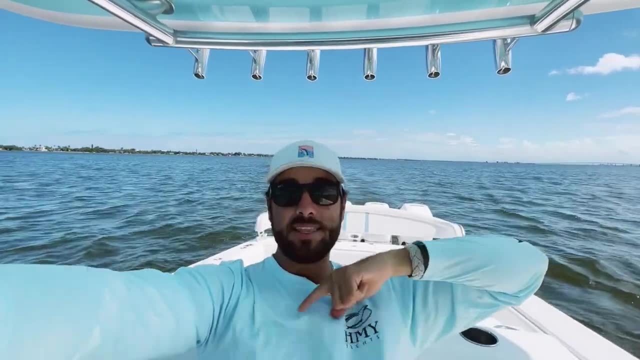 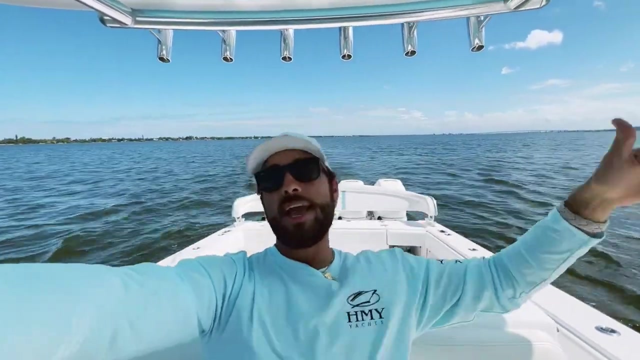 a saying: it goes red right returning. If you're returning into a marina, the red marker needs to be off the right side of your boat. If you're returning from the ocean into an inlet, the red marker needs to stay off the red side of your boat. If you're coming into anywhere and you're coming back into, 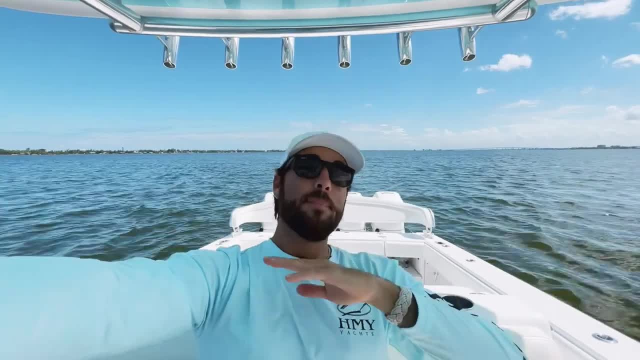 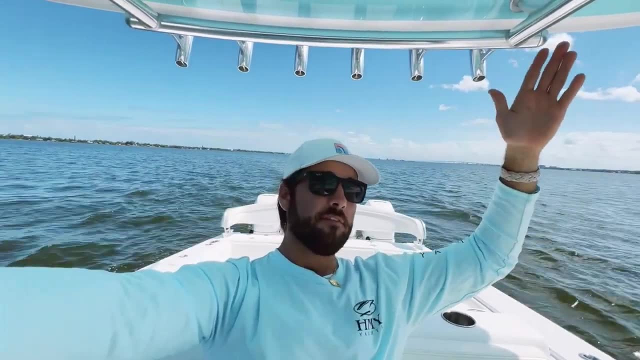 that marina, that port, that harbor and there are channel markers. Make sure you keep the red marker off the right side of your boat And you know, inversely, the green marker stays off the left side of your boat. You need to stay in between the red and green markers. 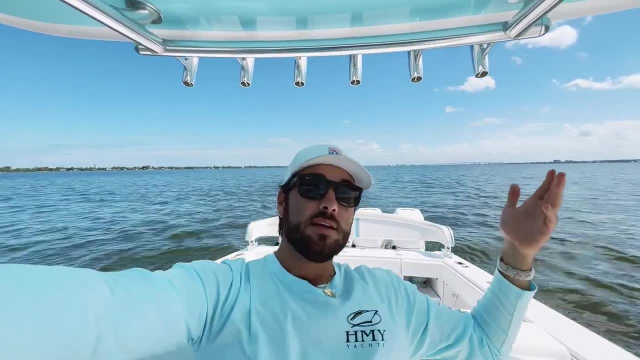 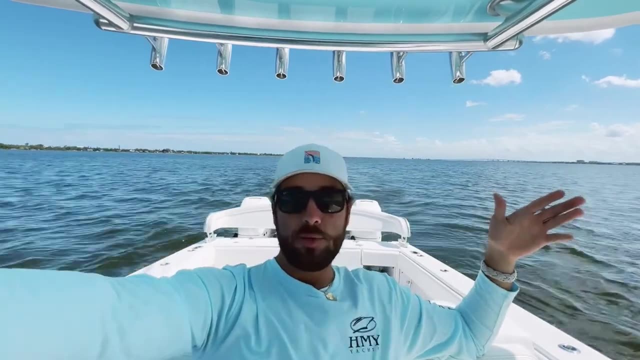 red off the right side, green off of the left side. You know, right starboard, left port. It's pretty simple: when you come in and out of places, Stay between the buoys, the red and the green buoys. 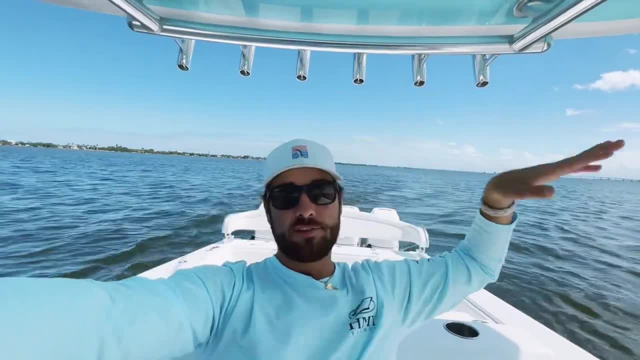 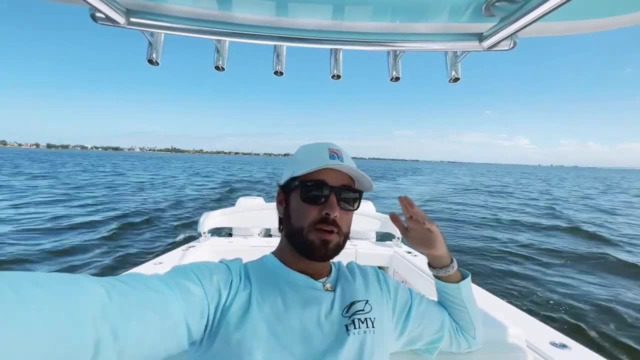 The red one needs to stay off the starboard or right side of your boat. The green one needs to stay off of the left or port side of your boat. They mark the deep water. they mark the channel that is safe for navigation, the deep water channel. stay between them. 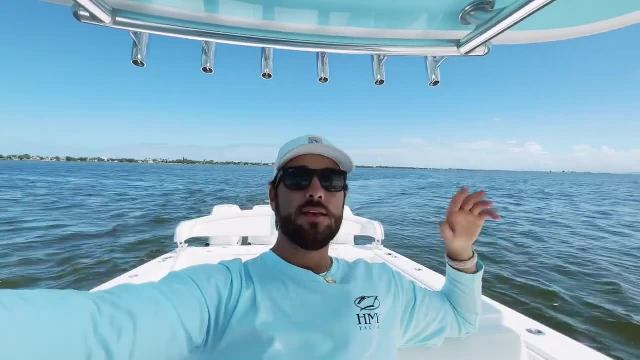 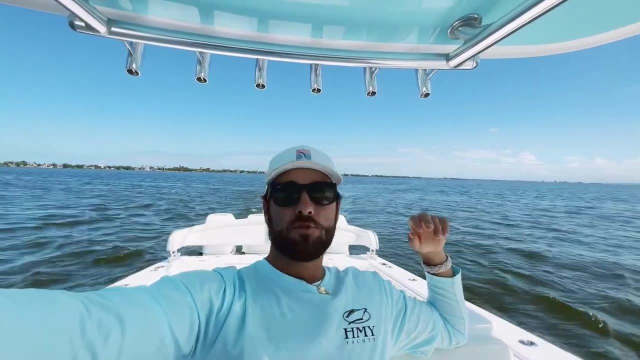 If there's a marked channel, stay in it. It's the safest way to do it And know that you keep the red marker to your right side and the green marker to your left side: Red to starboard, green to port, red, right returning. 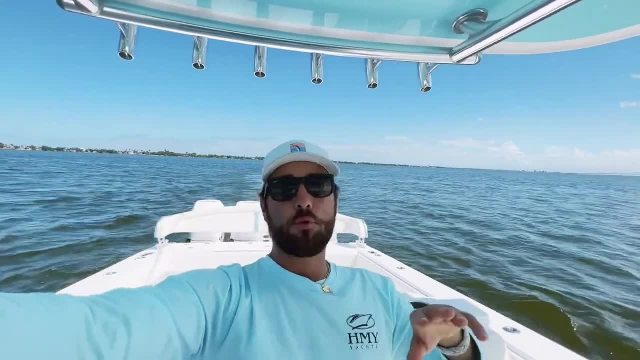 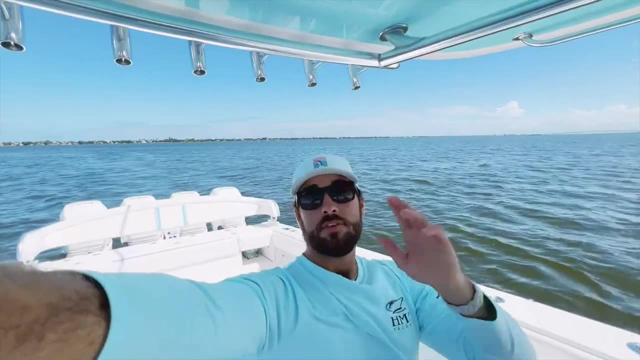 Know that rule, memorize it, never forget it. It's the most important thing that you can know when it comes to navigating a boat safely in and out of ports, inlets and marinas. The next thing you need to know is when you're navigating. 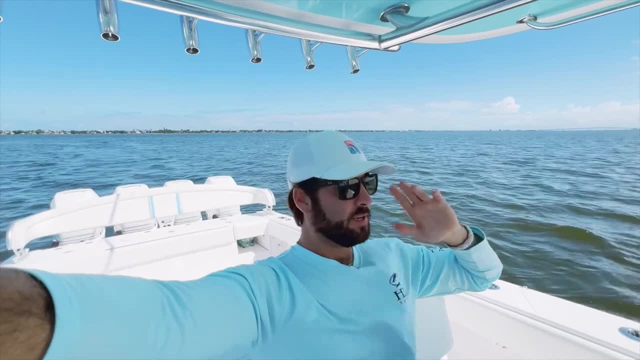 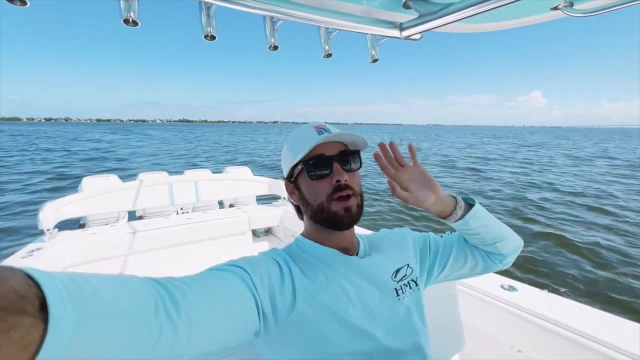 a boat in the intercoastal- This is gonna be 99% of boaters who this video reaches. who is in Florida? the inland waterways, inland rivers, they have a completely different set. This is for intercoastal boaters. 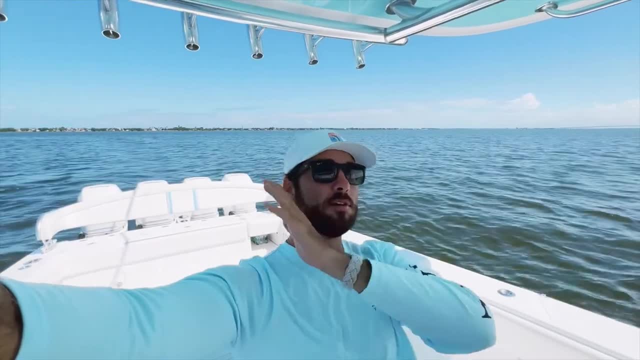 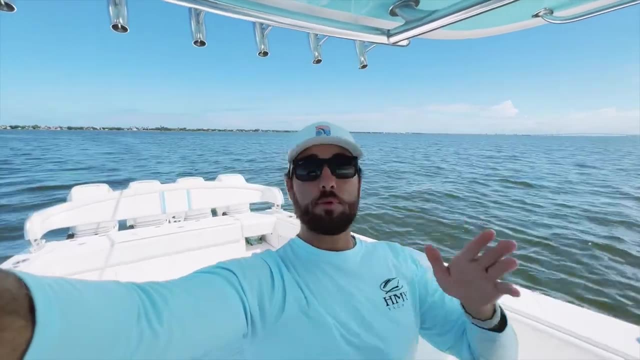 Rule of thumb: if you're heading south in the intercoastal, the red marker stays on your right side, The green marker stays on your left side In the intercoastal. it's very important to stay in the channeling parts because they can get pretty shallow. 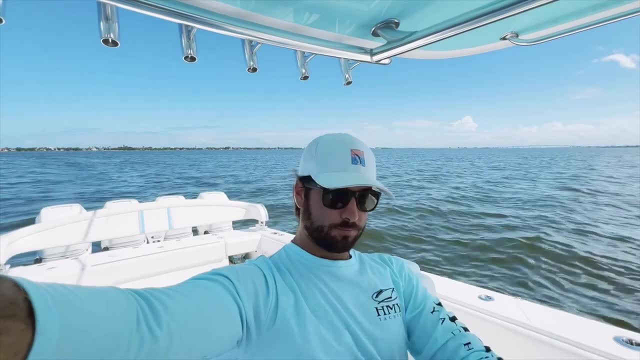 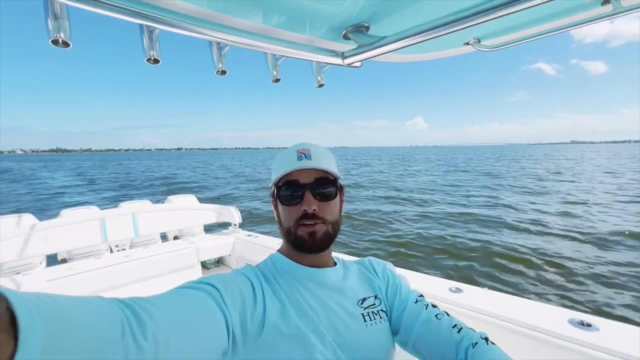 especially in parts like central Florida Melbourne Bureau north of there, Especially once you're at Titusville Mosquito Lagoon. You know, stay in the channel. The green stays on your right side If you're heading north, if you're heading south. 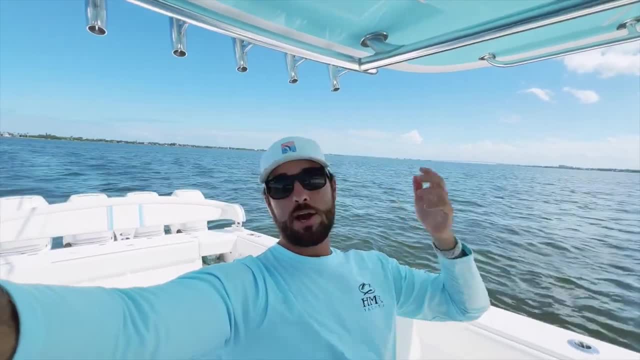 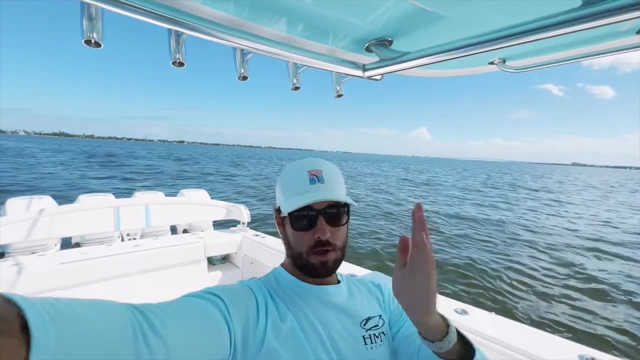 the red stays on your right side. There's really no rhyme or anything to remember it. Just know that if you're heading south in the intercoastal, the red marker stays on your right side, your starboard side, and the green marker stays on your left side, your port side. 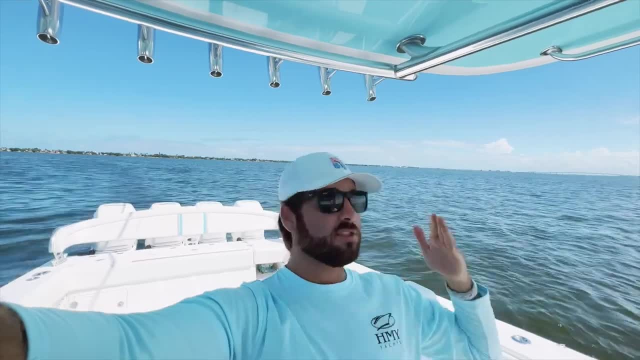 And of course, it's inverse: if you're heading north, the green is going to be on the right, the red is going to be on the left. Here's actually a channel marker right here. I'm in the intercoastal of Melbourne right now. 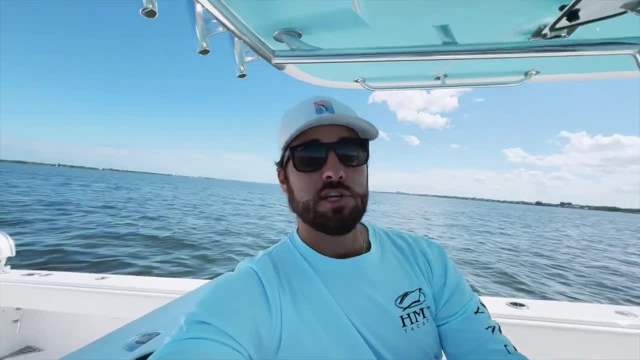 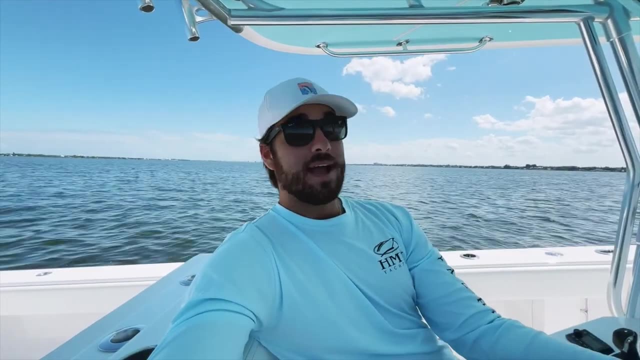 You can see it's a square. One thing you'll notice too is all the green channel markers are squares and the red ones are triangles. That's another way that you can identify it. If you can't see the color, know the shape. 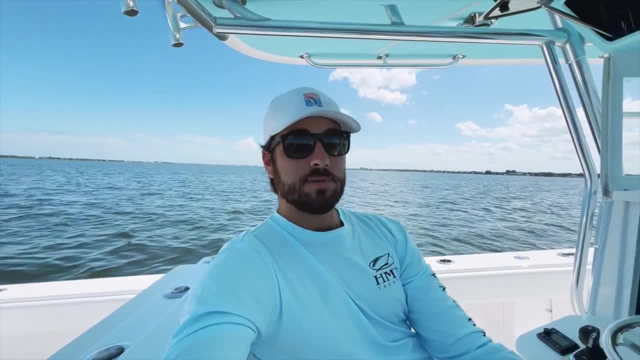 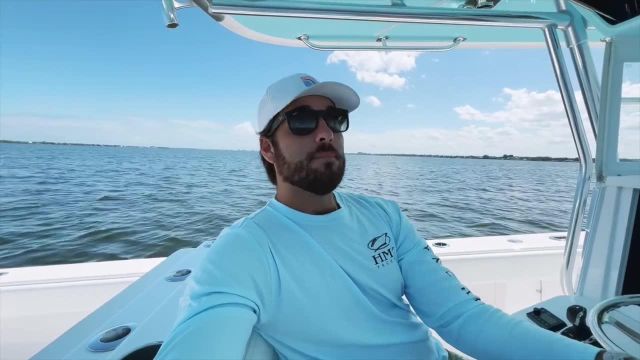 You know, the red ones will always be triangles, The green ones will always be squares. There's also a yellow square On there. I don't know if you can see. that's the shape you're supposed to look at and abide by. 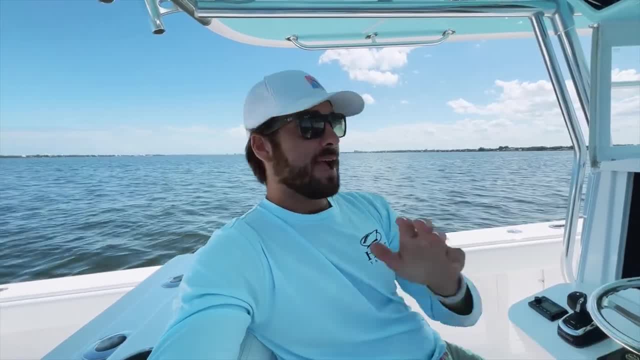 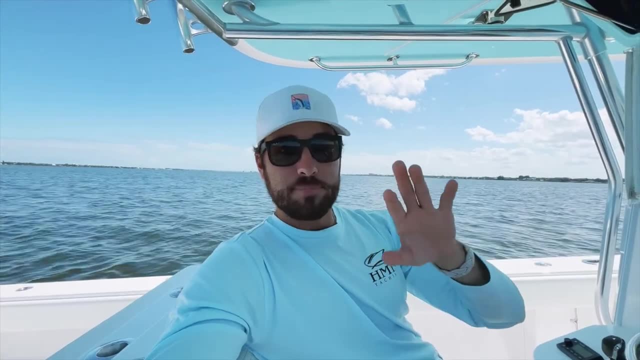 And channel markers are number two and there's a rhyme and a reason for the numbering. However, that's while important to know, it's not important to know for the everyday. you know. new boater For them. just know red should be on your right side. 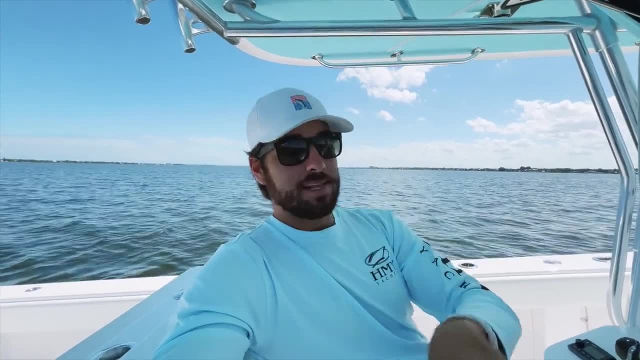 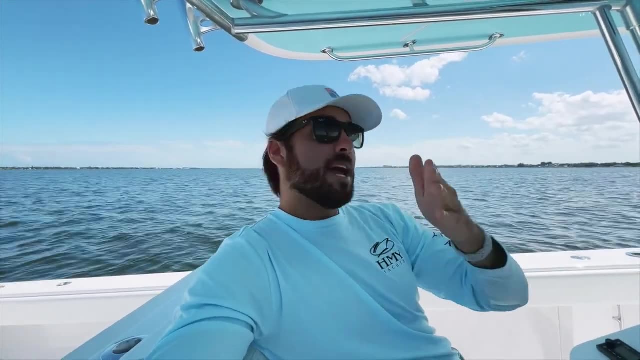 coming and going, returning to any port: Red on your right, green on your left. If you're leaving the port, the green on your right, red on your left. If you're going up and down the intercoastal south, the red's gonna be on your right. 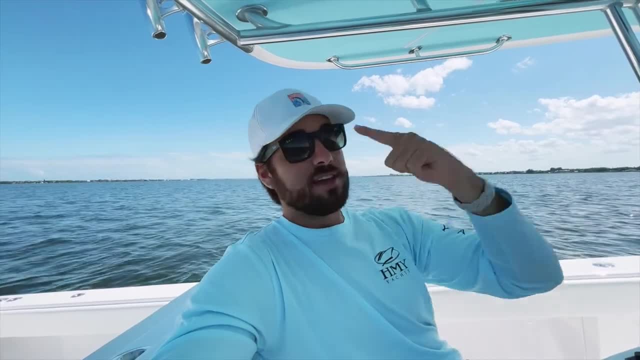 the green's gonna be on your left. If you're heading north, the green's gonna be on your right. the red's gonna be on your left. Those are just rules that you have to memorize. There's nothing else to it. 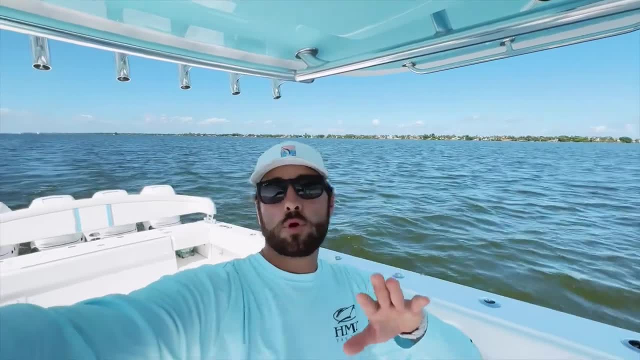 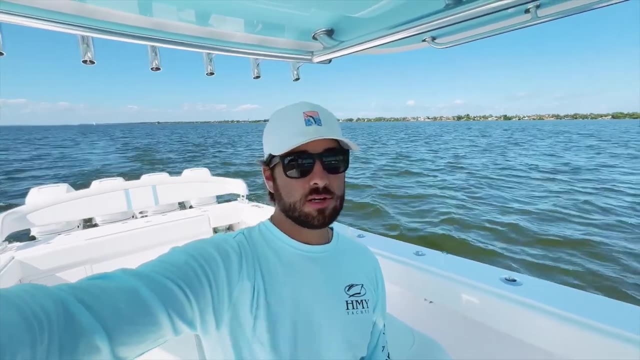 Memorize them. it's the safe way to navigate. And one more quick thing to mention is that there are different kinds of navigational markers. You will occasionally see different kind of channel markers, but for the most part for the everyday boater. 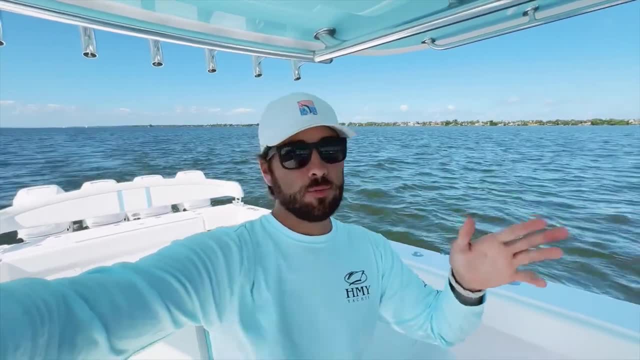 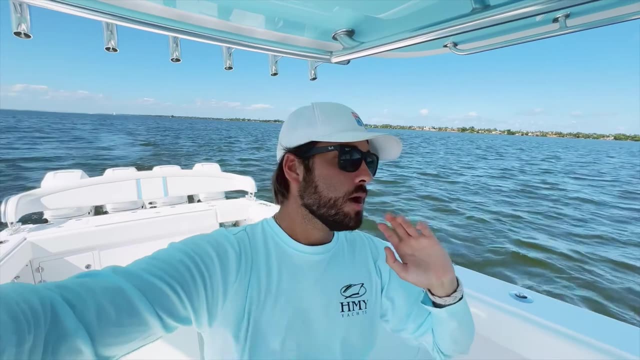 you don't have to know that stuff. If you see it, just kind of go by it as you normally would. If you see a big sign, the red circle on it, slow down. Sometimes it might be a no but no motor zone. 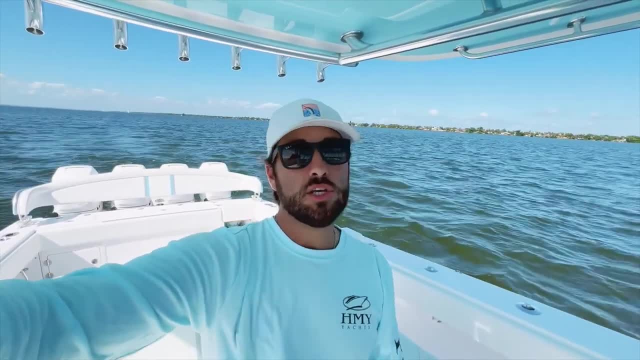 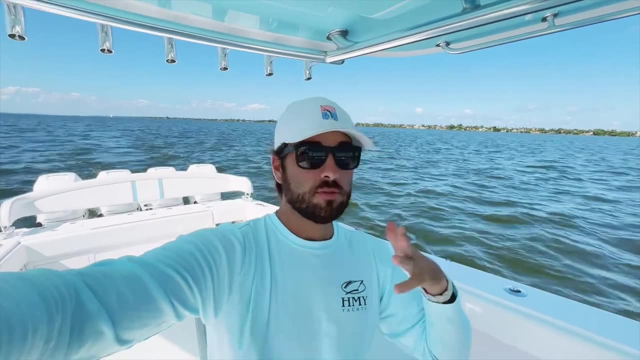 And then the only other one maybe- is occasionally coming into ports. you will see a channel marker, which will be in the form of a buoy that is both green and red, both And that's the case. You can safely pass on either side of that buoy. 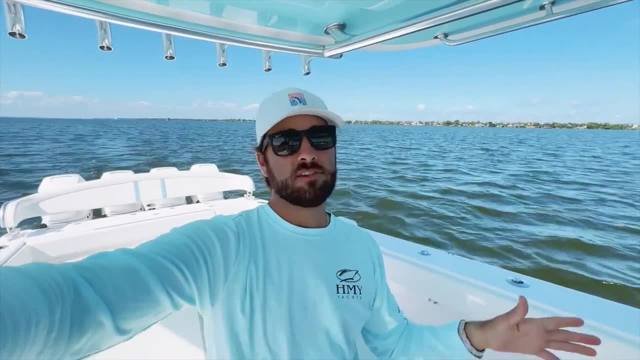 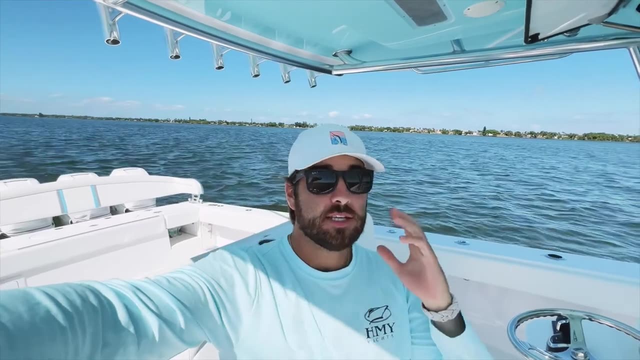 Besides that, all the other ones don't really pertain to the average recreational boater. You won't have to know that, And so the next and probably last topic that I'm gonna cover in this video is no wake zones and when you can safely go fast. 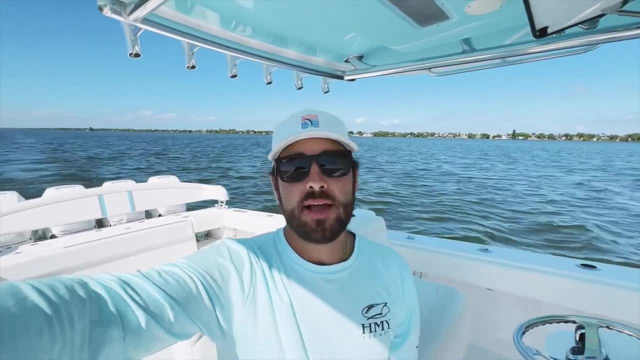 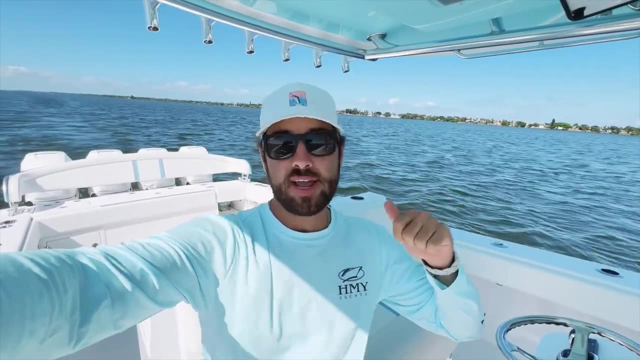 These are pretty visibly marked And there's also a sense of judgment that you have to use for this. You know, at the end of the day, you, as the operator of your vessel, you are responsible for the wake that your boat creates and any damage that that wake creates. 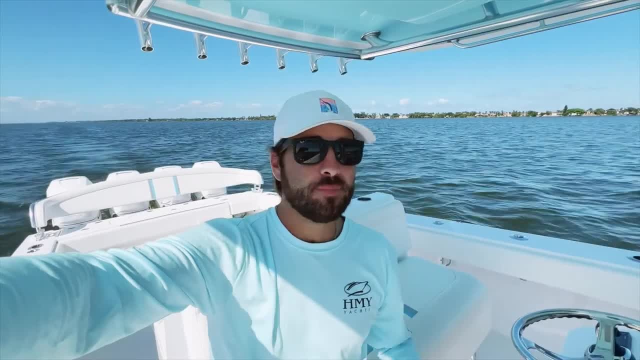 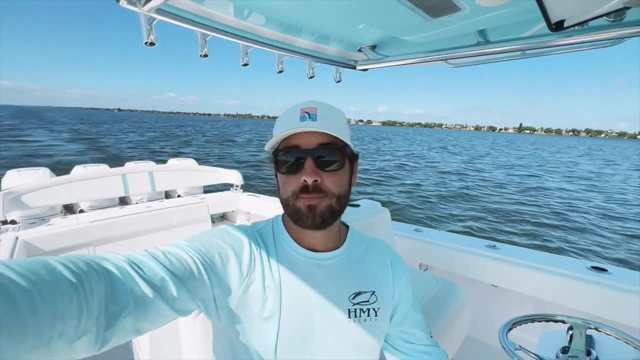 So be smart. If you're running right next to docks with a bunch of boats tied up, don't go super fast by them and make all those boats slam into the dock, because you are responsible for that. They will come after you and you're gonna have to pay for all the damage. 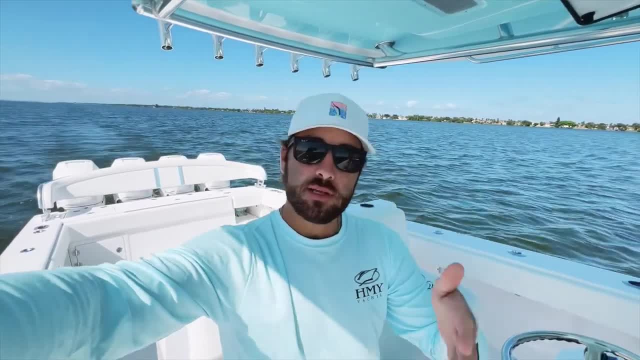 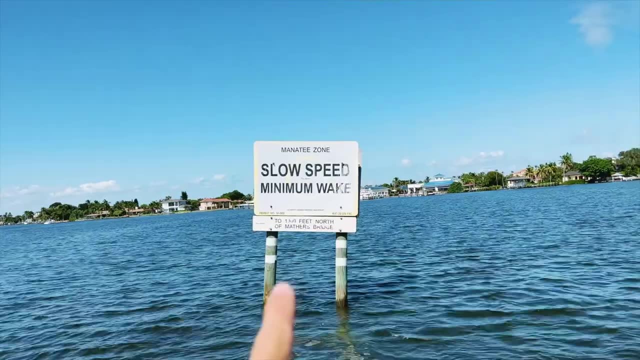 But generally speaking, no wake zones are pretty well marked. I'll show you what a no wake sign looks like. So this is what a no wake sign looks like. You can see. it's huge. It's very easily marked. It says slow speed, minimum wake. 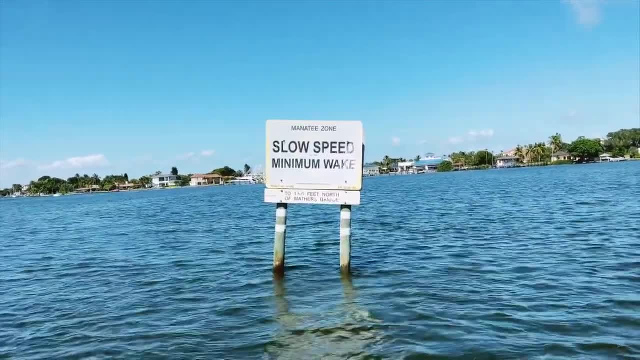 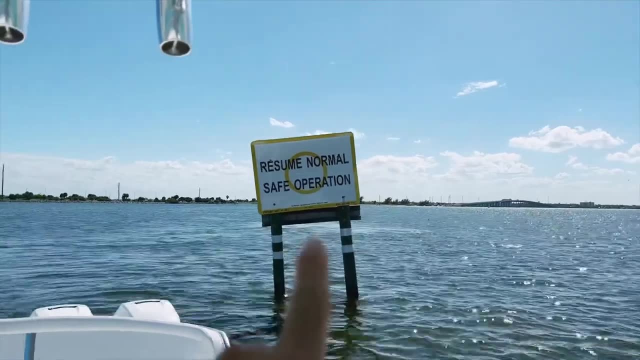 And then on the bottom there, it tells you until what point down the river. They're big, they're hard to miss. That's what they look like, And that is what the sign will look like when you're allowed to go fast again. 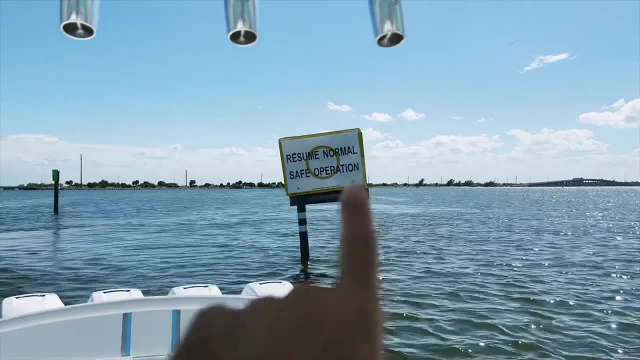 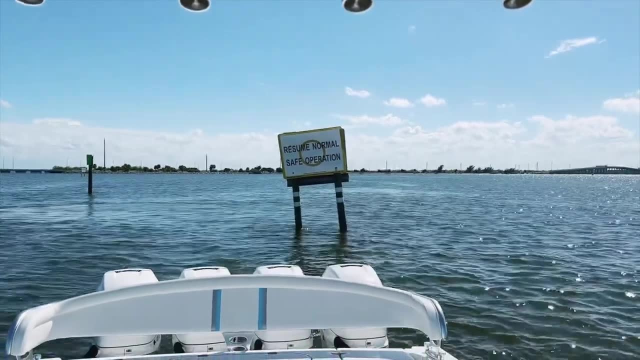 Again, it's big, You can't miss it. If there is a speed limit, it'll say it on the bottom of that sign. But when you're allowed to go fast on everything, this is the sign. Once you pass it, you're good to go fast. 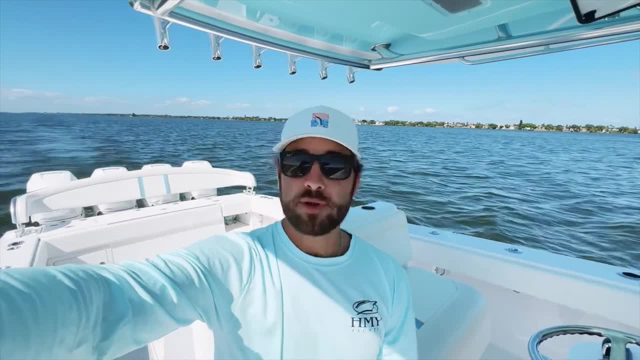 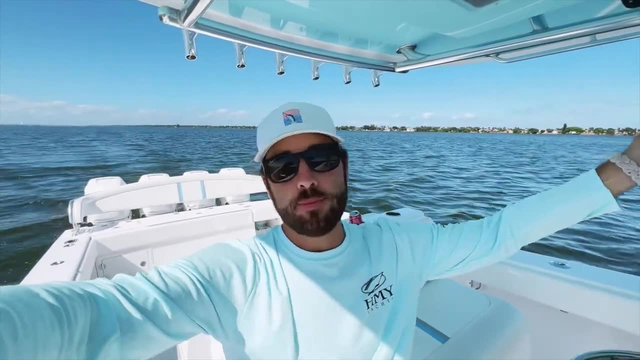 and do whatever you want to do, And in those zones do not bring your boat above idle. You know, if your boat's in neutral, move the throttles, one click forward and you're in idle. You're gonna, depending on the boat. 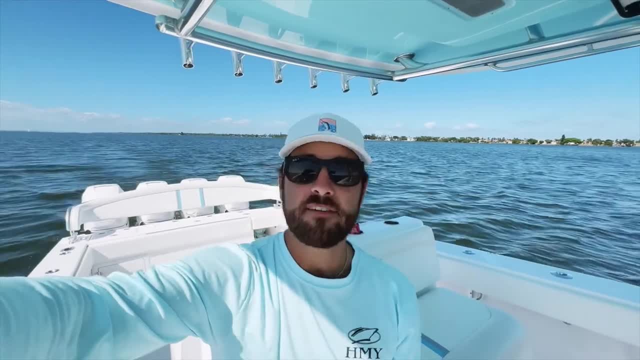 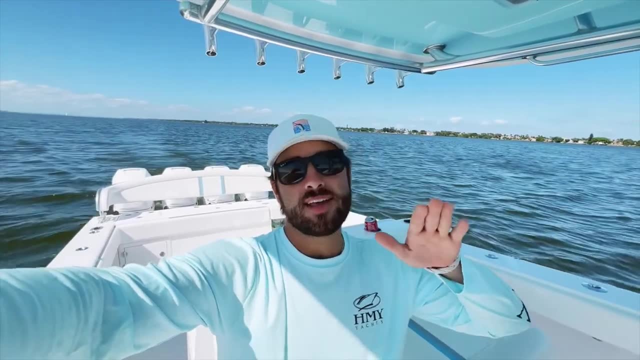 be going anywhere between two and a half to four, maybe four and a half miles per hour, And don't go fast in that. because once you start going fast in that, you know your boat kind of starts to slow down, It starts to plow. 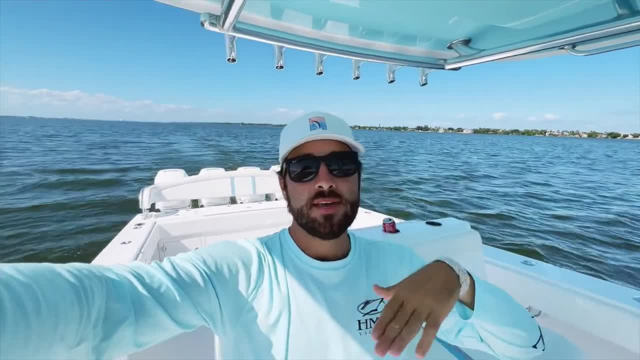 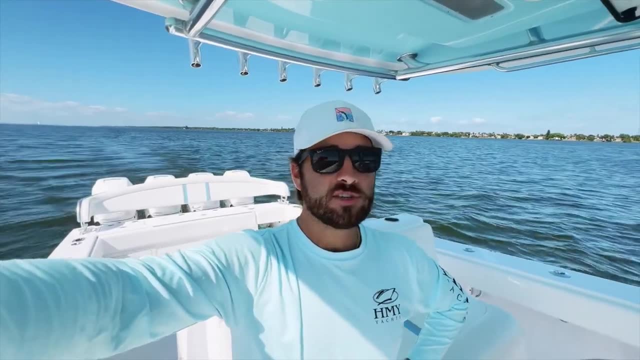 And that's where the back of your boat starts to kind of push down. your bow goes up and you're creating a huge wake, even a bigger wake than you would be if you're going fast in a lot of situations, And it's dangerous. 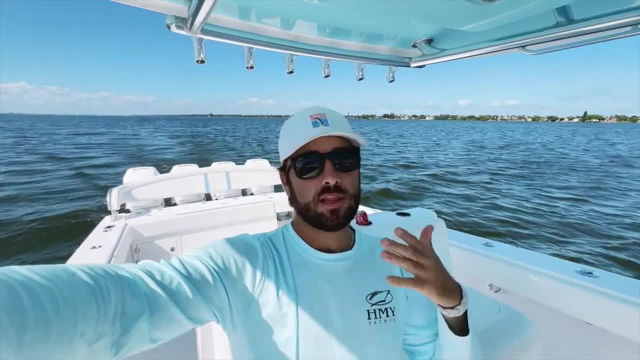 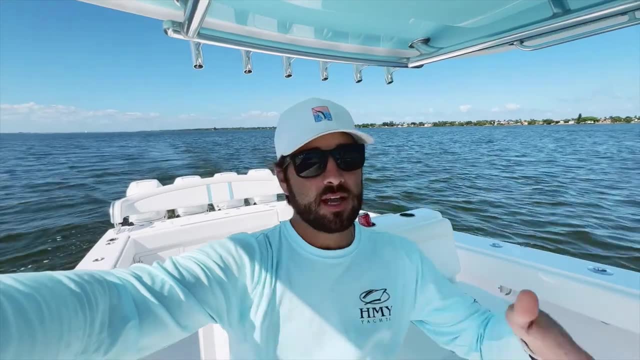 You know there's a reason no wake zones are there. It's usually in crowded areas with a lot of boats tied up- residential areas, You know, if they don't want a bunch of boats coming through, making a bunch of wakes, slamming boats tied up into the docks. 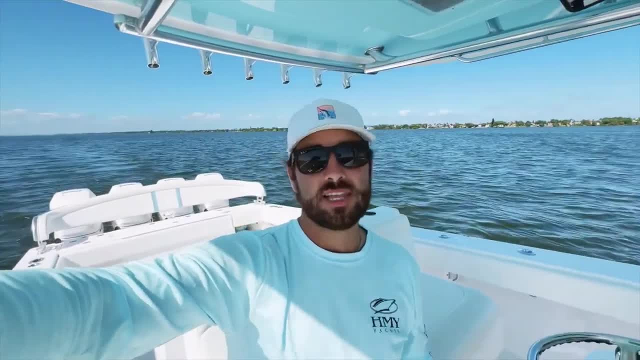 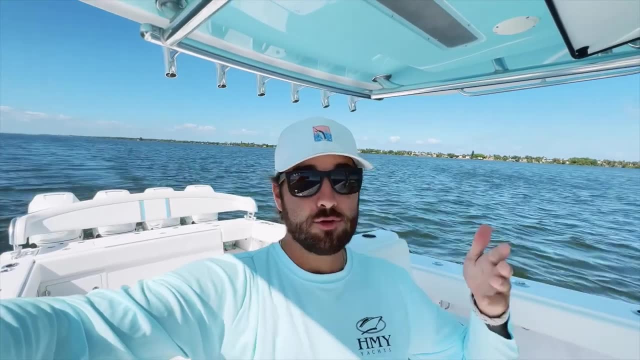 If you're going by a marina, you don't want to be slamming those boats into each other, slamming the boats into the pilings. So use some reason. If you're by that stuff and you're questioning whether you should be going fast or not, go slow. 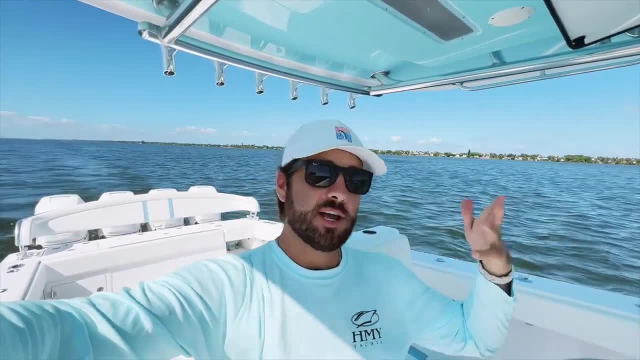 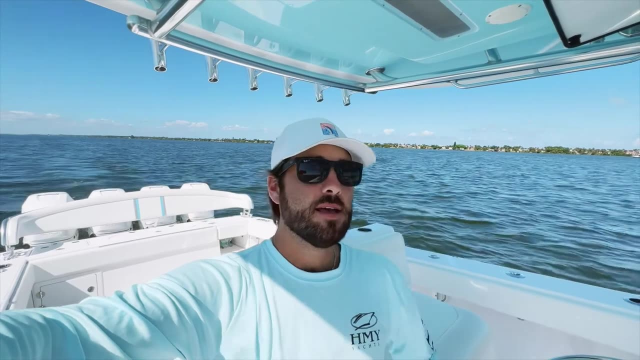 If there's any doubt, go slow. But the signs again I'll show you. they're pretty well marked. Go idle speed, you know. two and a half to four knots is going to be your best bet there, And don't go any faster. 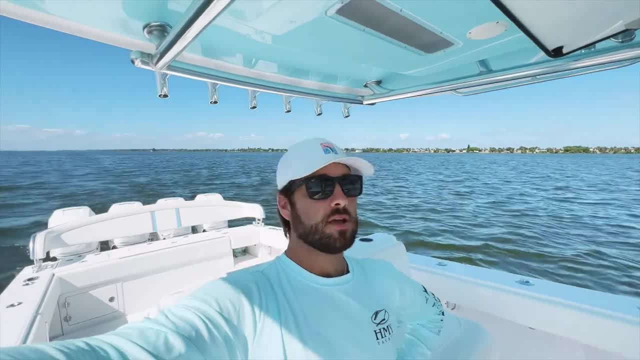 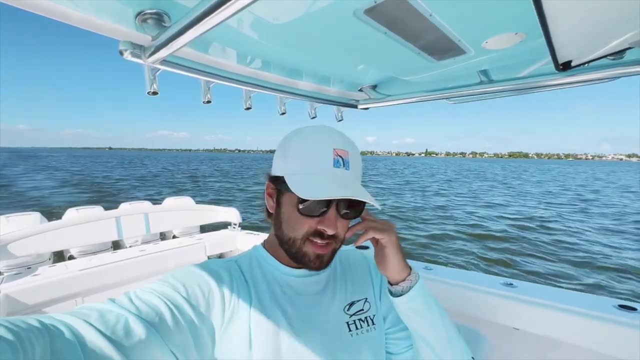 And the other reason is for manatees, especially here in Florida. You know manatees are. I don't think they're a danger anymore. I think they're actually on the threatened list though, But still you know they have a tendency. 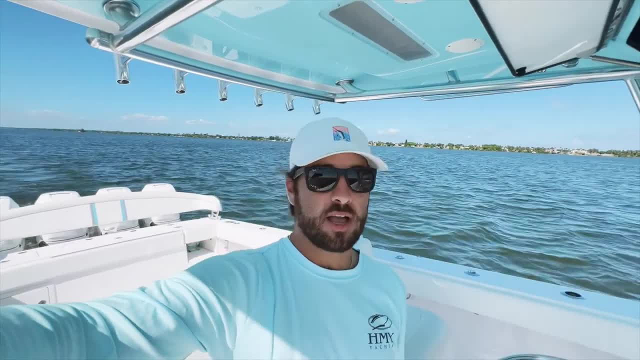 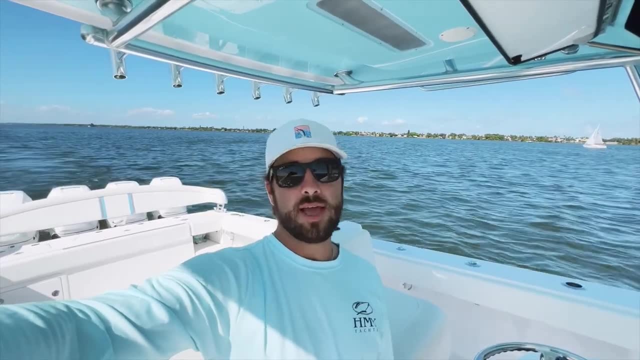 to get hit by boats because they're pretty stupid animals, and this except there when boats are coming. So if you're in shallow water you'll see a manatee sign. it'll say: you know, idle speed, minimum wake. do that, you know. 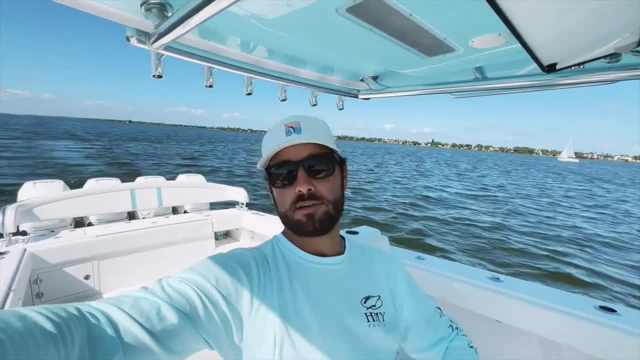 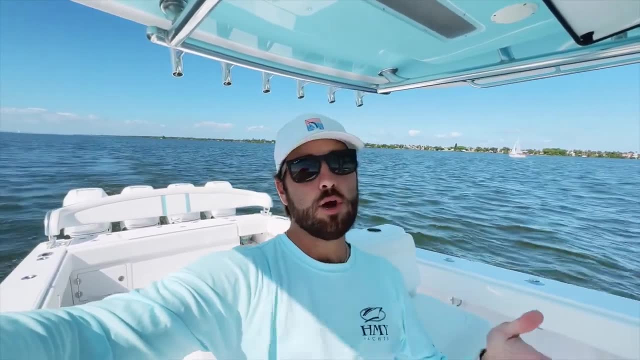 In those areas it's going to have a channel marker, probably every quarter mile, or it's not a channel marker, a no wake zone, probably every quarter mile or so surrounding that flat. So just be cautious of that, Know your waters, know where those no wake zones are. 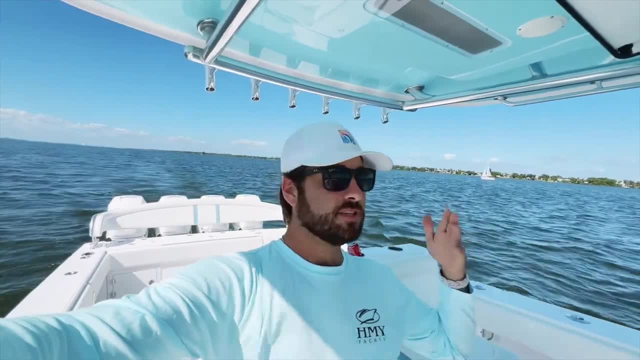 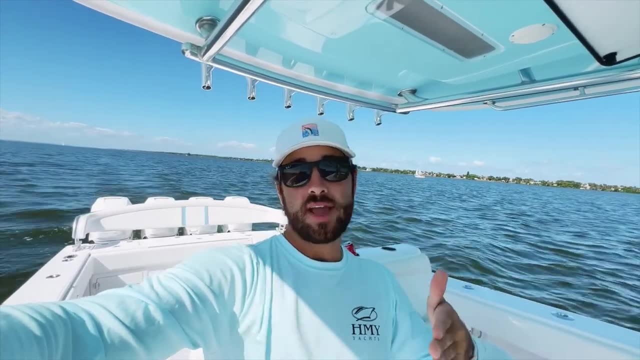 know where the manatee zones are And just use some common sense. If there's a bunch of boats tied up, if you're passing a marina, if you're going by a bunch of residential docks, be courteous, be slow, because if your wake causes damage, 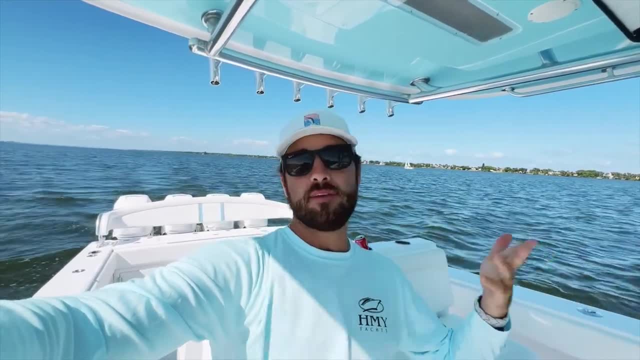 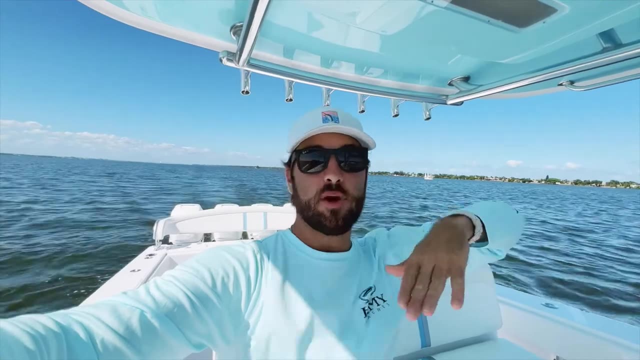 you are going to be the one paying for that damage When you're in open water. yeah, fine, go fast. You know, if you're in part of the intercoaster where you're allowed to go fast and all the houses along the sides have boats up on lifts.